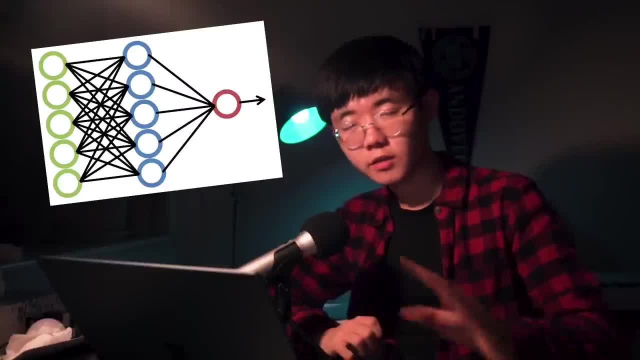 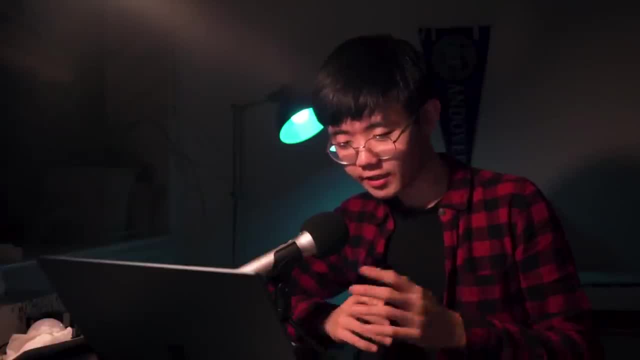 very familiar with neural networks at a high level. right, You have lots of layers, lots of nodes. you connect them all together. you can have some really complex models from it that make some some cool predictions, right? I find that a lot of that kind of learning, right when you're just 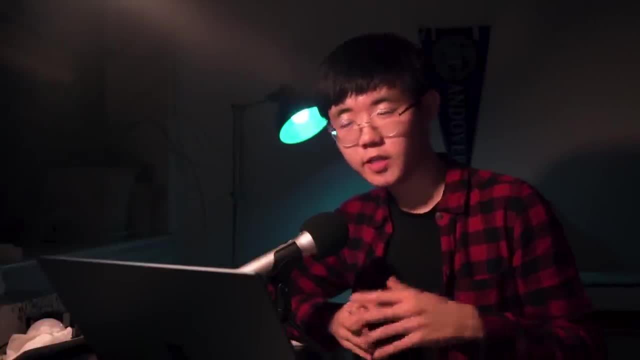 looking at stuff from the high level is kind of wishy-washy And even if you go into TensorFlow and implement these networks, it's still a little unclear, like how they work. you know, at least for me. I feel like I learn a lot better when I can get to the equations, when I can really build from. 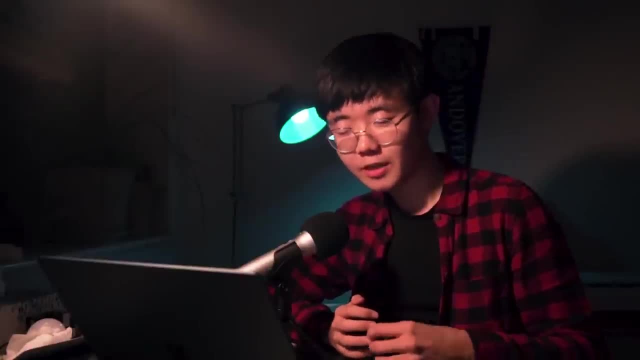 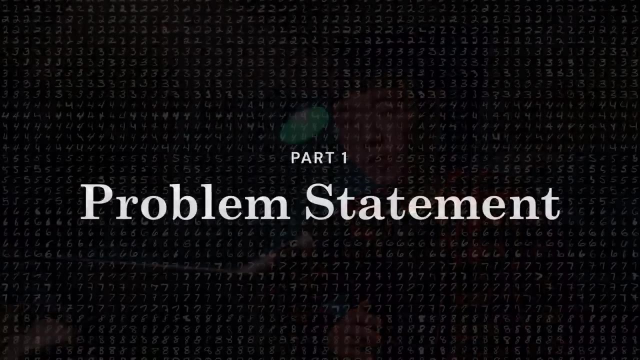 the ground up, and you really can't get too much closer than implementing a neural network from scratch. So that's what we're going to be doing today, So let's dive right into it. The problem that we'll be tackling is digitization. 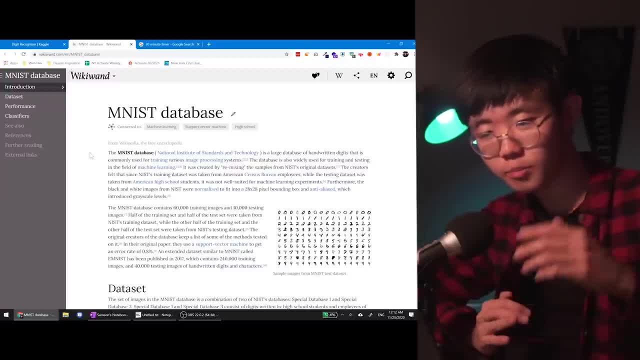 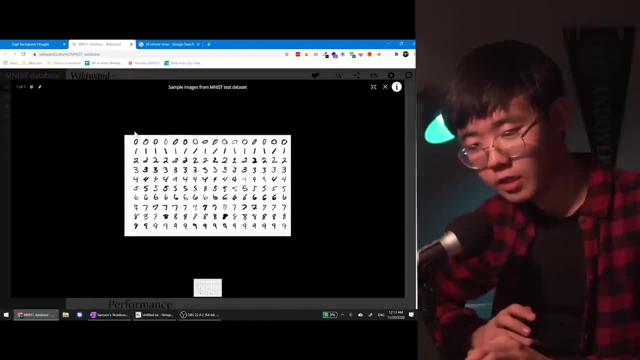 We'll be using a famous data set called the MNIST data set. So what the MNIST data set is is it's tens of thousands of these 28 by 28, so pretty low res, grayscale images of handwritten digits. We are going to be building a neural network that classifies images of handwritten. 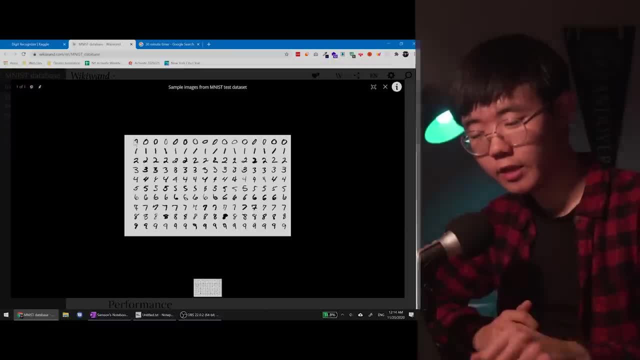 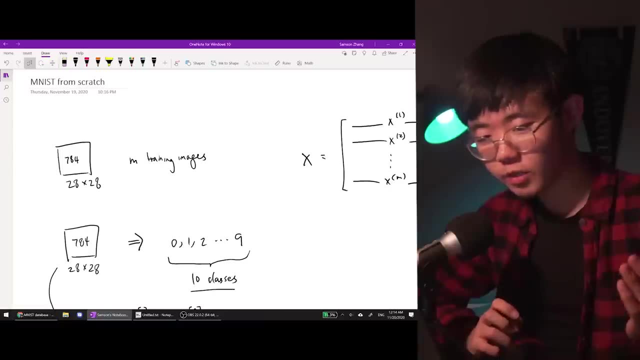 digits and tells you what digit is written in that image. This is an overview of what everything is going to look like, what we're going to implement today, And we're going to start off with 28 by 28 pixel training images, So that's 784 pixels overall, And each of those pixels is just 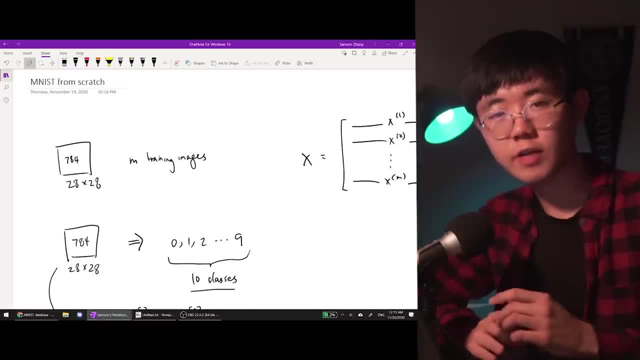 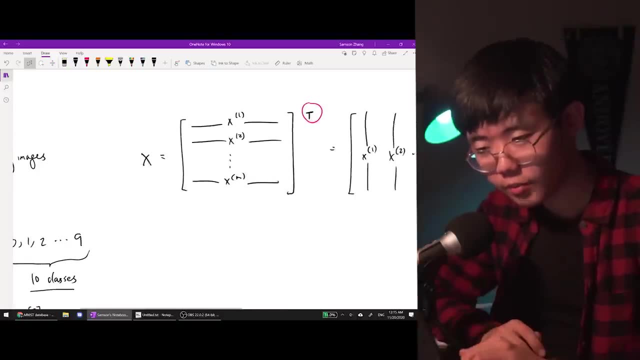 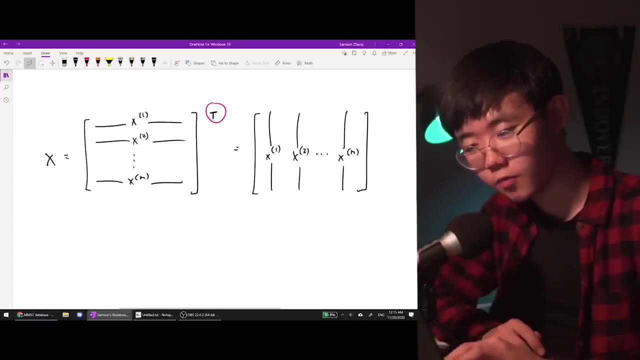 a pixel value, right, It's between zero and 255,, 255 being completely white, zero being completely black. So we have M of these training image So we can represent it as a matrix that looks like this: Each row constitutes an example, and each row is going to be 784 columns long, because each of them 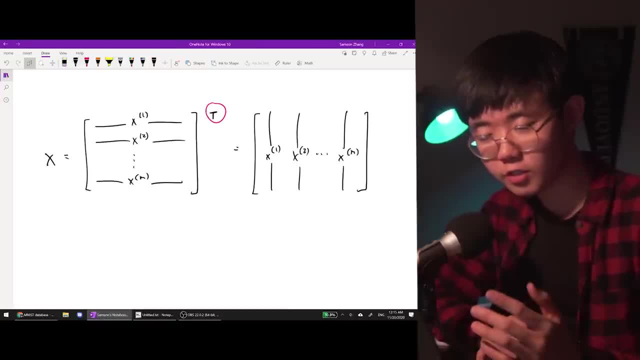 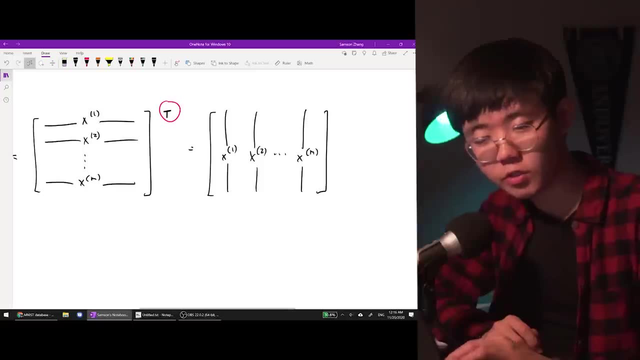 is going to correspond to one pixel in that image. What we're actually going to do is transpose this matrix. Instead of each row being an example, each column is an example. So our first column is going to be our first example, and it's going to have 784 rows corresponding to each pixel, And we're going to have M columns. 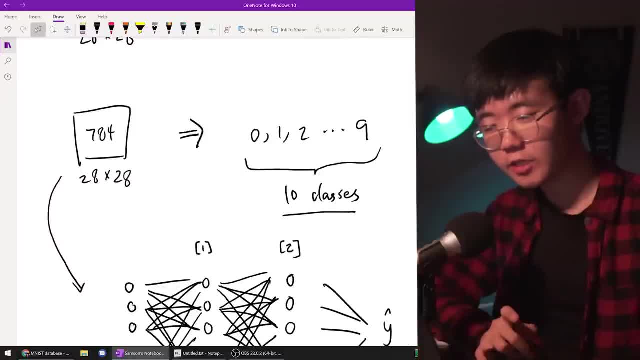 corresponding to our M training examples. Our goal is to take this image, just do a bunch of processing and then give out a prediction for what digit that image represents. And how we're going to do that is we're going to do a simple neural network, So we're going to be building a 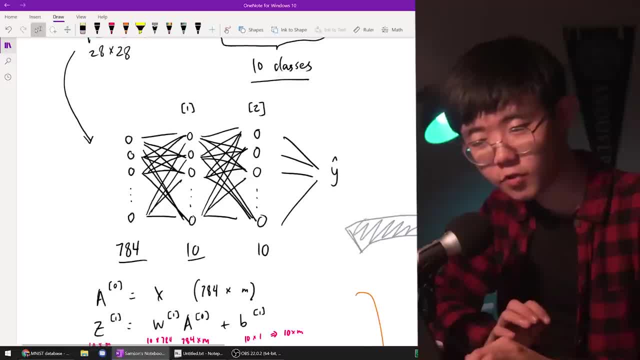 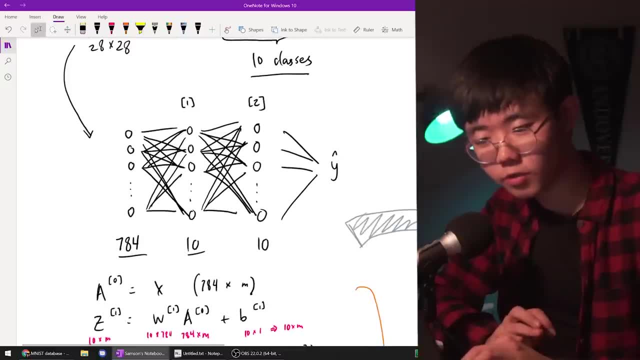 quite simple neural network. It's only going to have two layers, So the first layer in this neural network is just going to be 784 nodes. This is our input layer, right? Each of the 784 pixels maps to a node and that's our first layer. Our second layer is going to be our hidden layer and it's 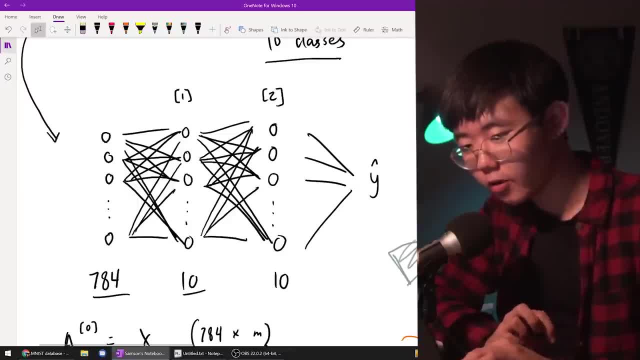 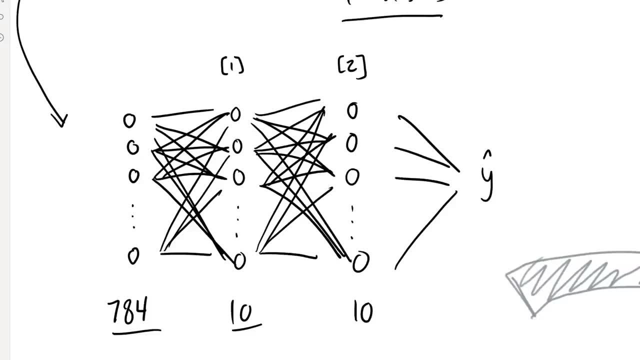 going to have 10 units And then our third layer is going to be our output layer, again with 10 units and each corresponding to one digit that can be predicted In that intro. right there, I called this the first layer, This the second layer and this the third layer. Going forward, I'm actually going to be calling 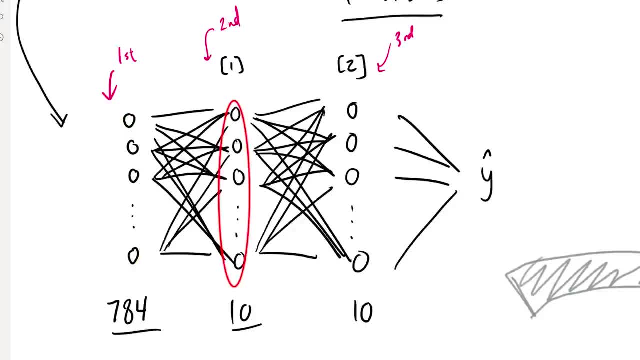 this right here, the zeroth layer, This the first layer and this the second layer. And the reason for that is this layer right here will also be called the input layer. There's no parameters here, right? This is not really a layer of the network, It's just the input. This right here is. 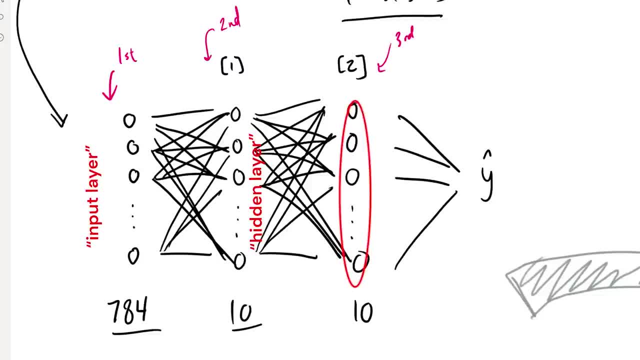 the first hidden layer, And this is our second layer and also our output layer. So yeah, so I just called them first, second and third layers, And then I'm going to call this the input layer. But going forward, we're going to be not using first, second and third, but rather input layer. 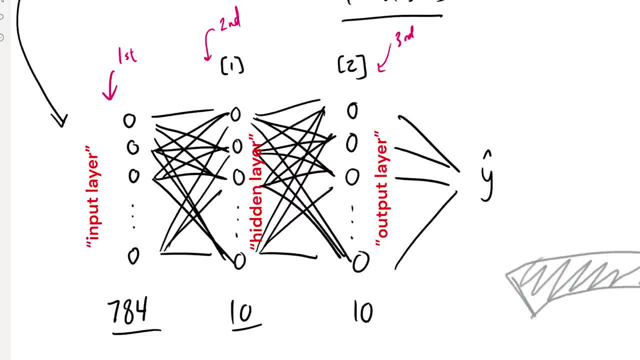 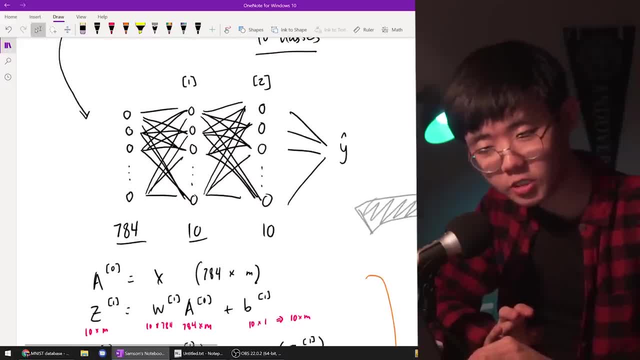 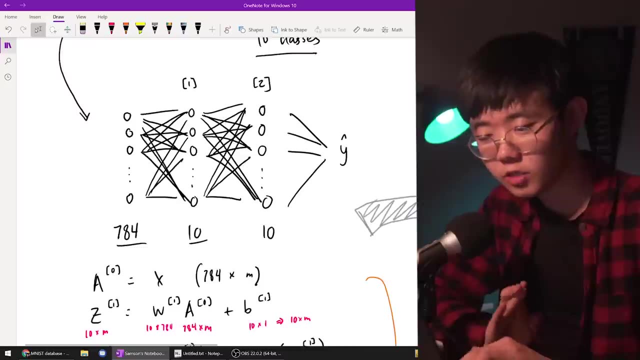 first hidden layer, and second layer, otherwise known as output layer. There's three parts to training this network. The first part is called forward propagation. So forward propagation is just when you take an image and you run it through this network. From this network you compute what your output is going to be. So that's the first part that we 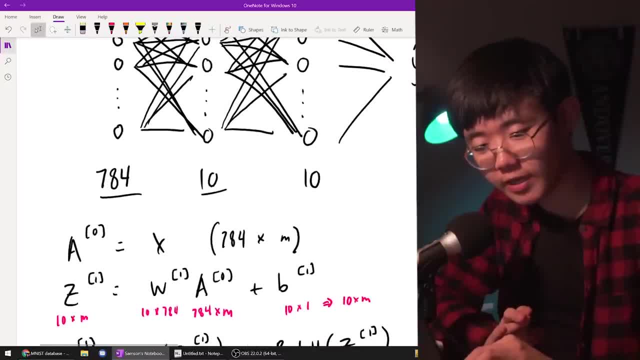 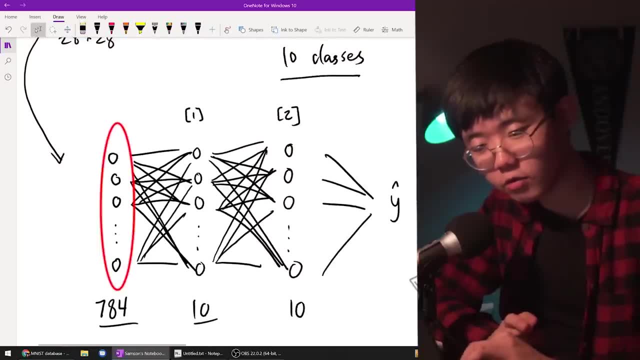 have to figure out. So to start, we're going to have this variable: a zero. That's just our input layer. That's just equal to x. There's no processing going on here. A zero is just this first layer, right. Z one is the unactivated first layer. What we're going to do to get z one is: 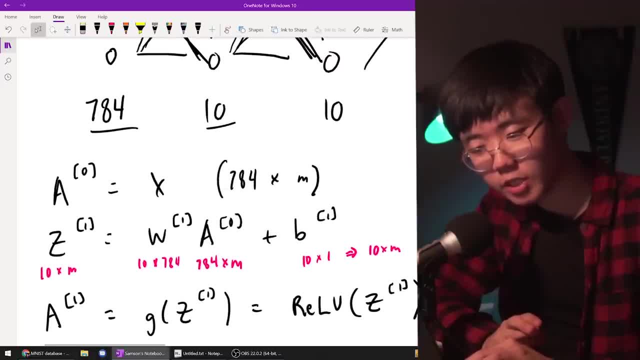 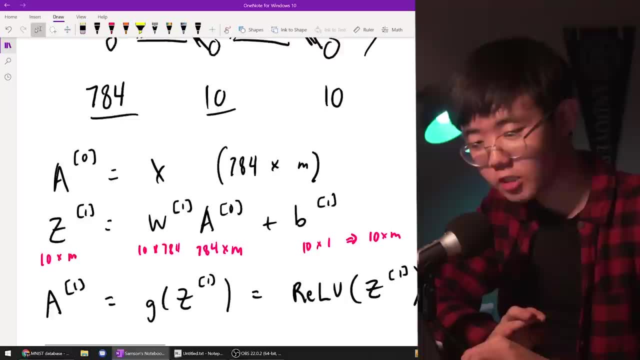 apply a weight and a bias. So a weight is going to be this matrix, We're going to take the dot product between that matrix and an, a zero, our input layer matrix, And that's going to give us something, and then we're going to add just a bias term to it. What we're doing here is really: 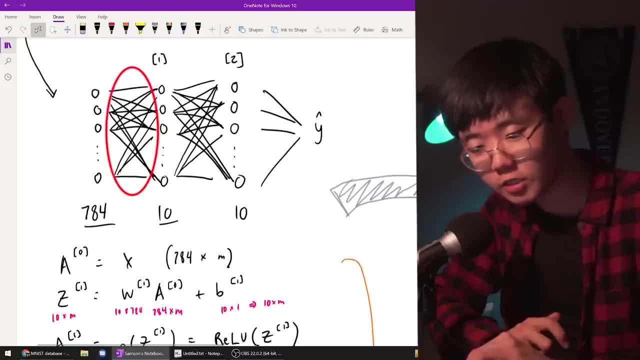 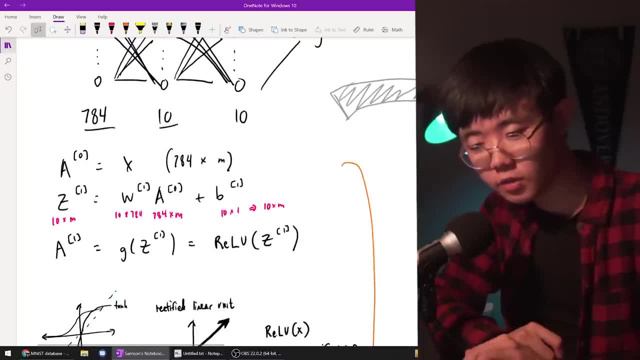 multiplying by a bunch of weights that correspond to each of these connections. Each of these, what? 7,840 connections? And then we're going to add a constant bias term to each of the nodes. What we're going to do after that is kind of interesting. We're going to apply an 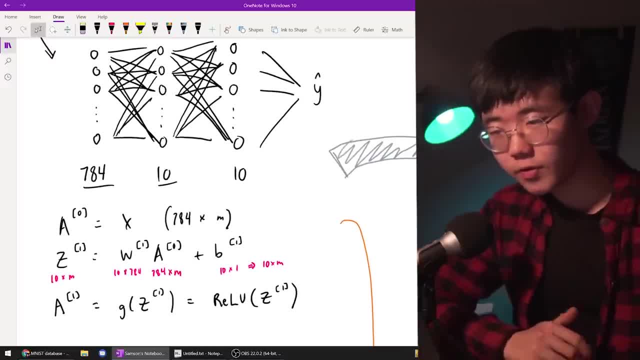 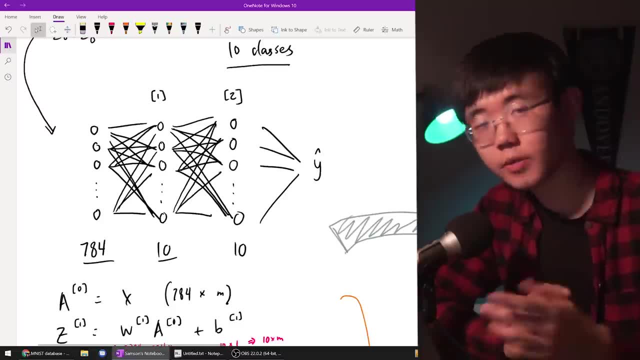 activation function to it. So if we didn't apply an activation function, what would happen is that each node would just be a linear combination of the nodes before it, right Plus a bias term. The second layer is going to be a linear combination of the nodes in the first layer. 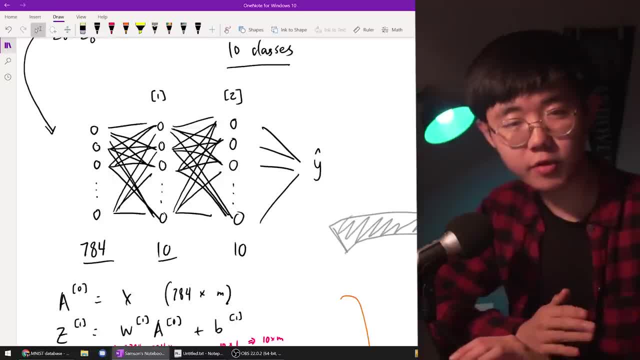 but the first layer is just a linear combination of the nodes in the input. So what's really happened is that that second layer is just a linear combination of the input layer. right, It's like you don't have a hidden layer at all. So if you only have linear combinations, 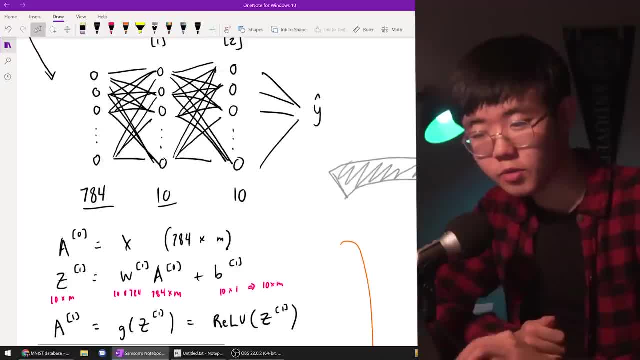 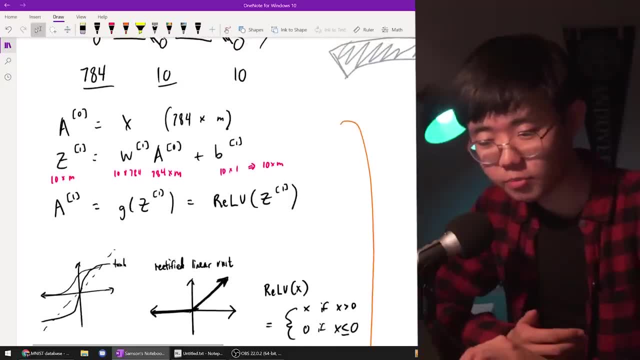 if you only have your weights and your biases, you're never going to get a really interesting function out of the neural network. Really, you're just doing a really fancy linear regression. To solve that, we apply a activation function. There's a bunch of common ones, so tanh and 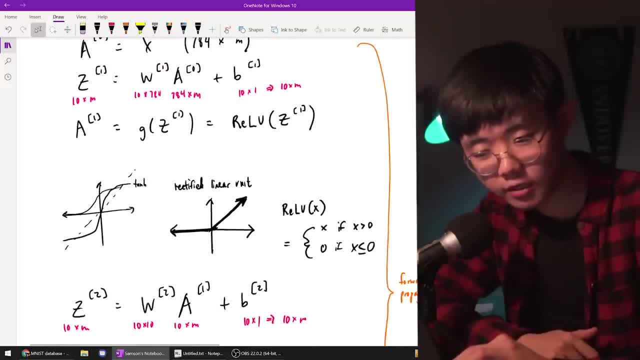 sigmoid. I'm sure you've heard of them. They kind of have a lot of different functions but they're going to look like this. You know, they got your nice curves and that's going to make it more interesting If you apply a tanh function or a sigmoid function to all of the nodes in a layer. 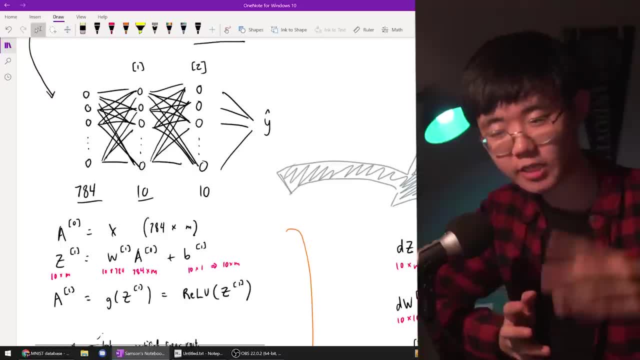 it's no longer linear, right When you move on to the second layer, that's adding now a layer of complexity and a layer of interesting nonlinear combination rather than just a linear model, And that's going to make your model able to be a lot more complex and more powerful. We're going to be 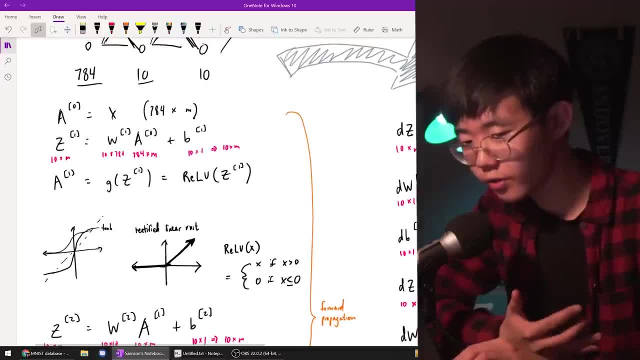 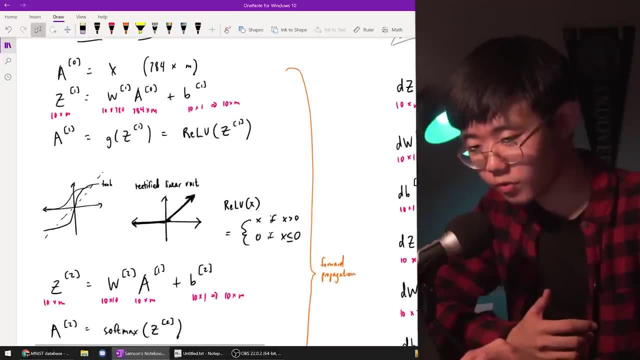 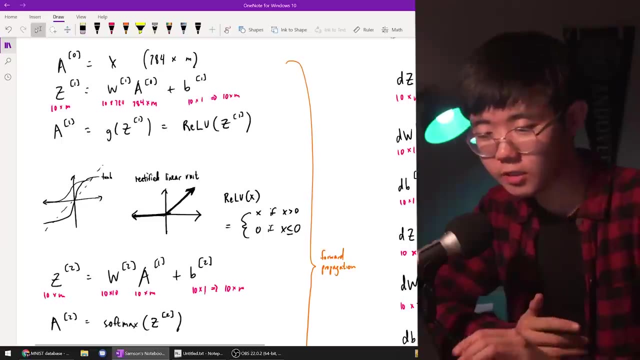 using another really commonly used activation function called relu or rectified linear unit. So relu just looks like this. It's really simple And how it works. so relu of x is defined as: if x is greater than 0, relu of x is just equal to x- It's literally linear- And if x is less than 0 or less. 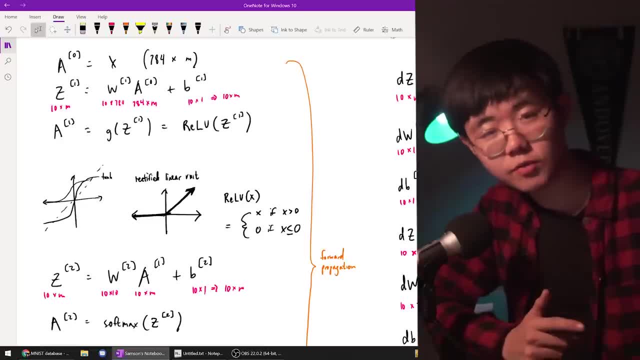 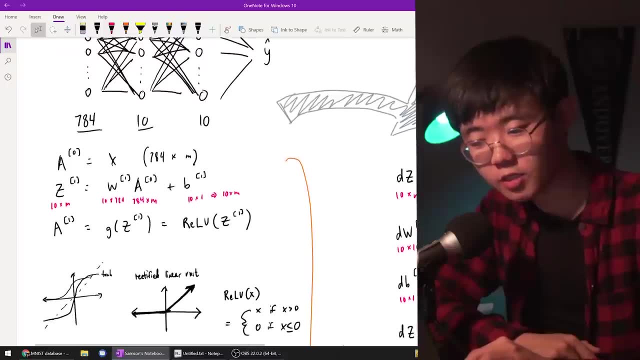 than or equal to 0,. it doesn't really matter, It's equal to 0.. Relu is equal to 0.. So it's just this really simple function, but just that's going to add the complexity that we need. a1 is going to. 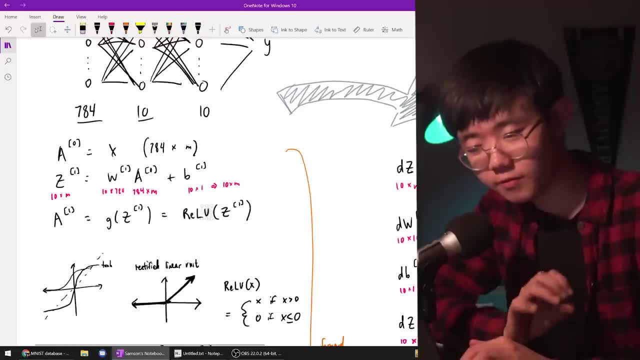 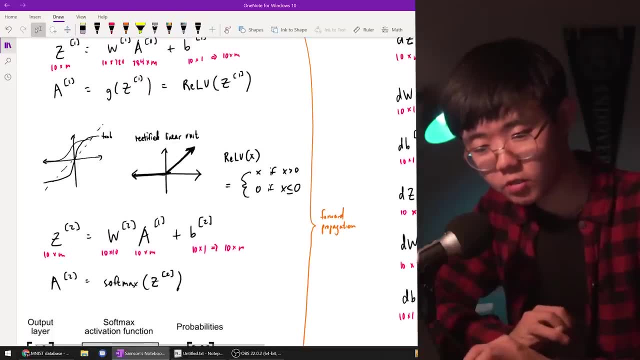 be equal to the relu function applied to every value in z1.. Now we're going to do kind of a test here and we're going to look at what we're going to get from layer 1 to layer 2.. So our z2,. 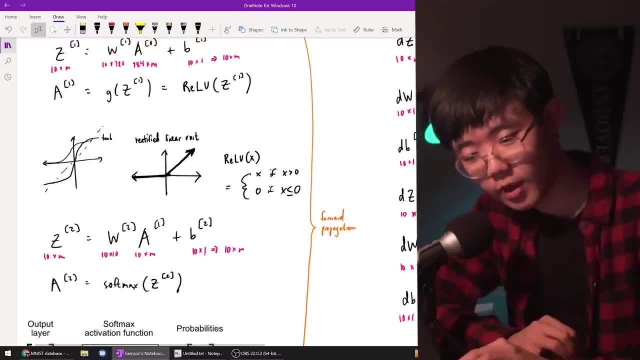 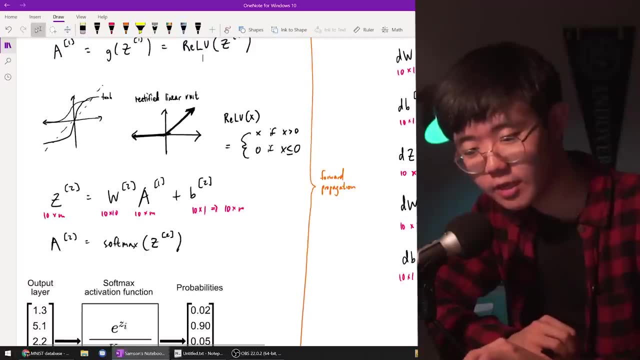 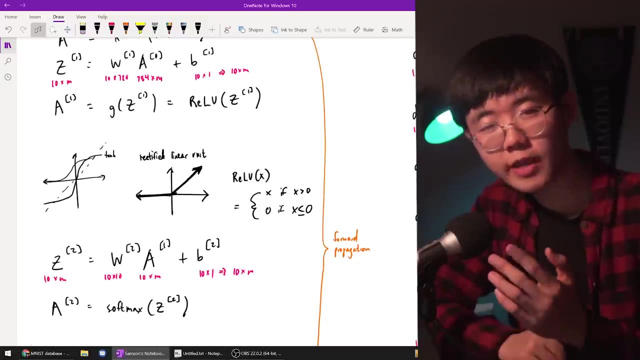 right. so our unactivated second layer values is going to be equal to a second weight parameter, right Weights corresponding to the values of the weights on each of these connections here between the first and the second layers, times our a1, times the activated first layer plus another constant. 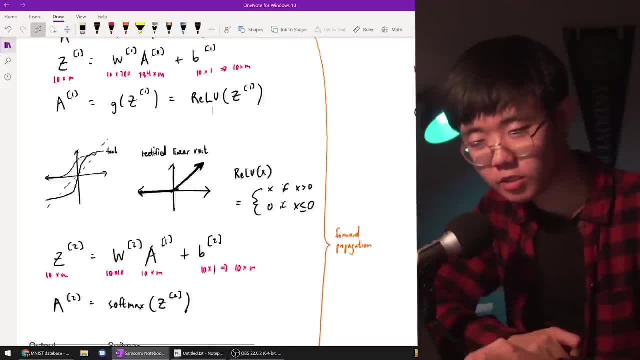 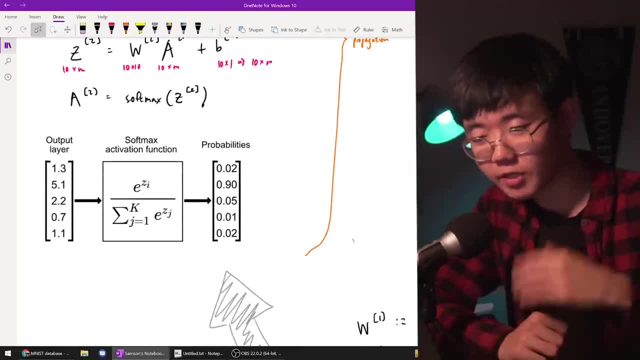 bias term. This time we're going to apply another activation function, but the activation function we are going to use is a relu or sigmoid or tantra or anything like that. It's going to be something quite different. It's called softmax Because this is an output layer right each of the 10 nodes. 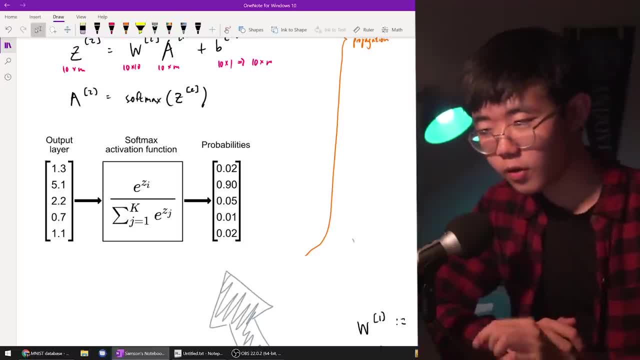 corresponds to each of the 10 digits that could be recognized. We want each of them to have a probability right. We want each of them to be a value between 0 and 1, where 1 is absolute certainty and 0 is no chance that that's what it is. So to get that, we use a softmax function. 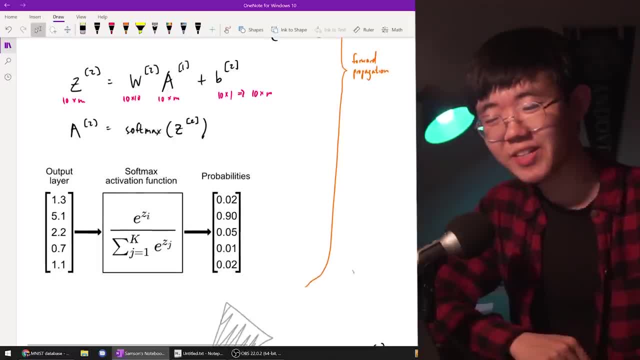 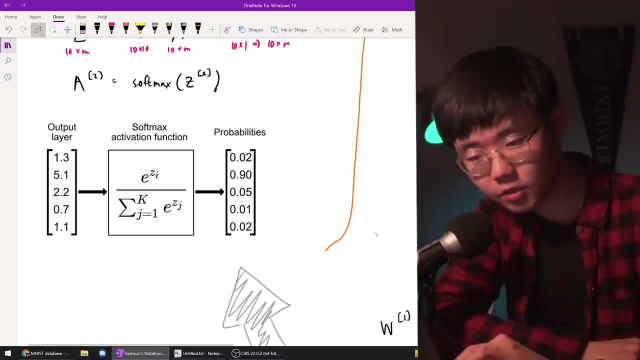 So I've just copy-pasted an image here. I didn't feel like writing this out myself. so it takes each of the nodes in the layer that you feed into it and it goes e to the z. so e to that node divided by the sum of e to all of the nodes right, Or rather the sum over all. 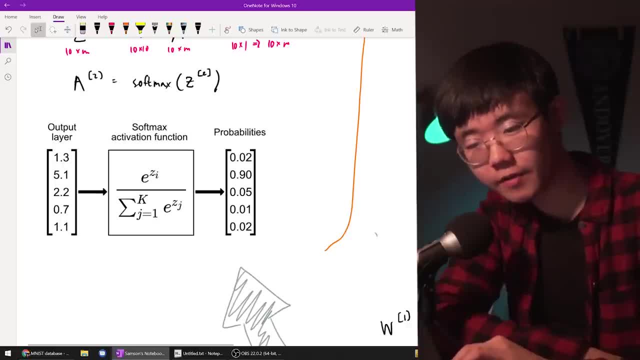 of the nodes, of e to that node, Each of your outputs after the softmax activation is going to be between 0 and 1, right, Because e to a single node is always just going to be a part of the whole. that is the sum of e to all the nodes. So for propagation is how you take an. 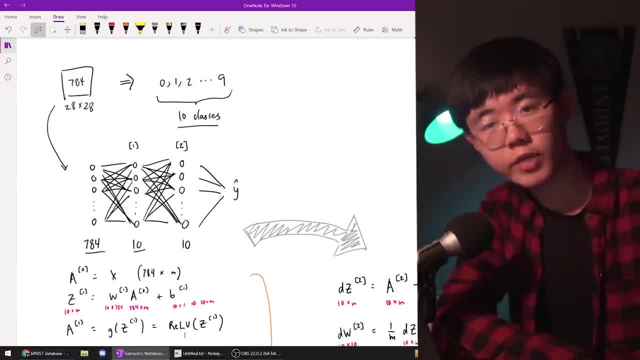 image and get a prediction out, But that's not enough, right? We need good weights and biases to make these predictions, And the whole thing about machine learning is that we will learn these weights and biases right. We will run an algorithm to optimize these weights and biases. 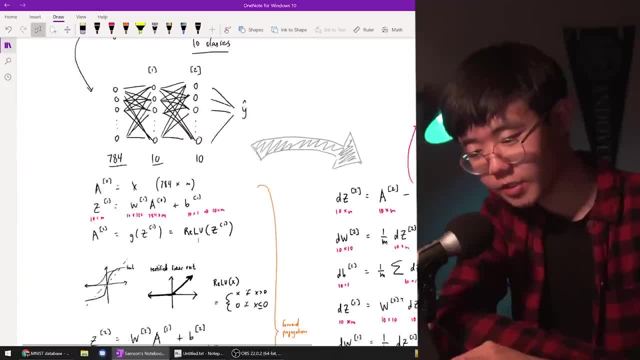 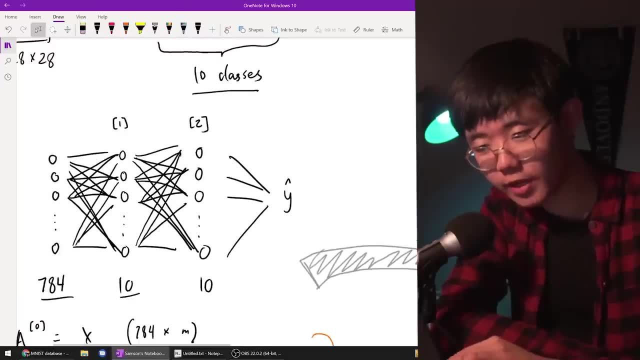 as we run it over and over again. We're going to do that in something called backprop, backwards propagation, And what we're doing here is basically going the opposite way. So we're going to start with our prediction and we're going to find out how much the prediction 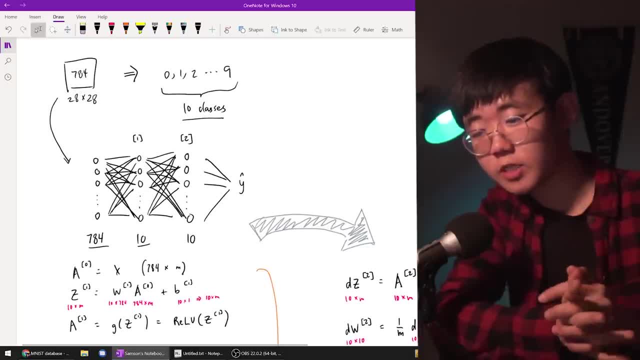 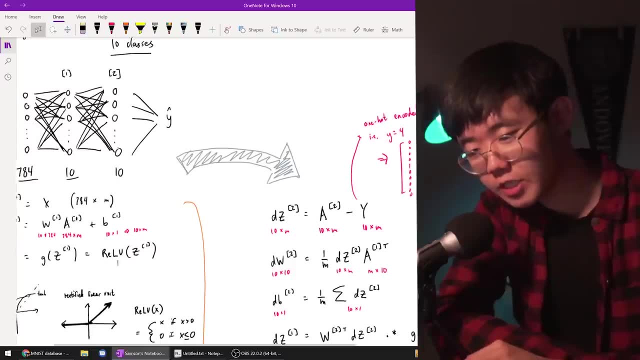 is going to give us an actual label, right. So that's going to give us a sort of error And then we're going to see how much each of the previous weights and biases contributed to that error And then we're going to adjust those things accordingly. So dz2 represents sort of an error of. 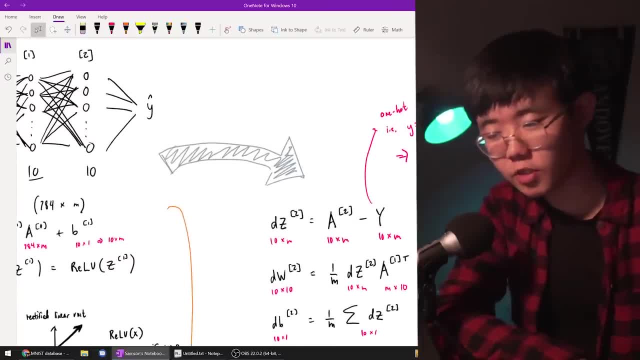 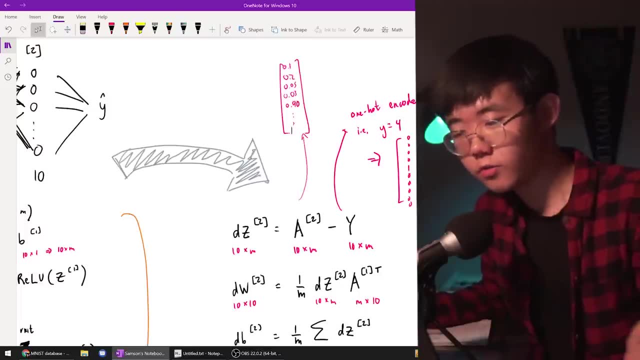 the second layer, right, It's how much the output layer is off by. And this is really simple. We just take our predictions and we subtract the actual labels from them And we're going to one hot encode the correct label. So, for example, if y equals four, we're not going to subtract four. 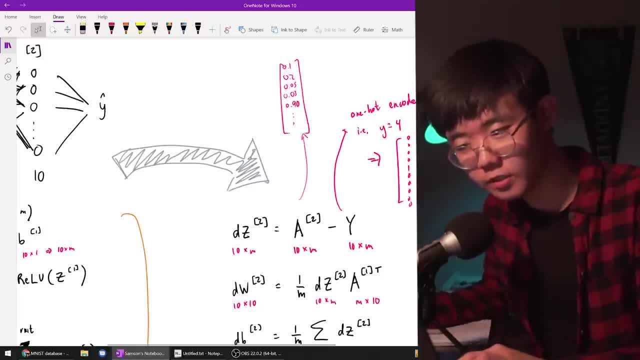 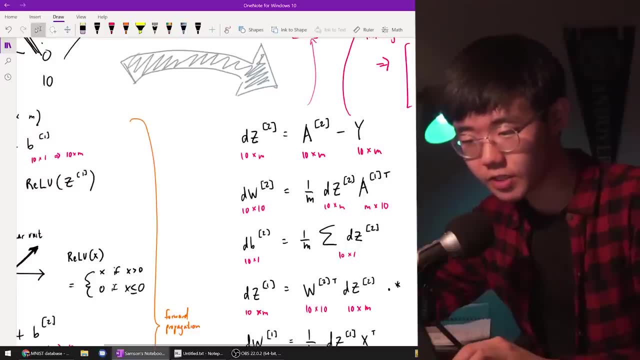 from this right We're going to encode: y equals four and we're going to subtract the actual four into this array. here, What are? the fourth index right Representing the fourth class is a one. Everything else has a zero. From there we do some fancy maths to figure out how much. 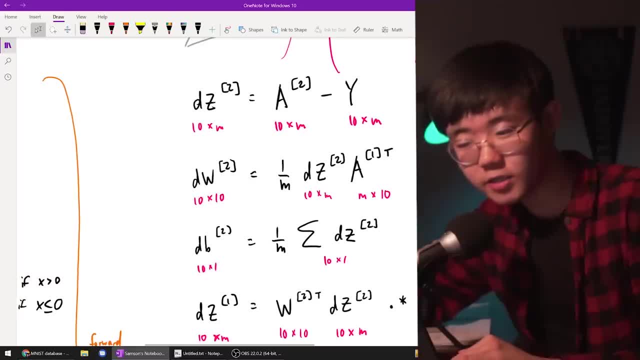 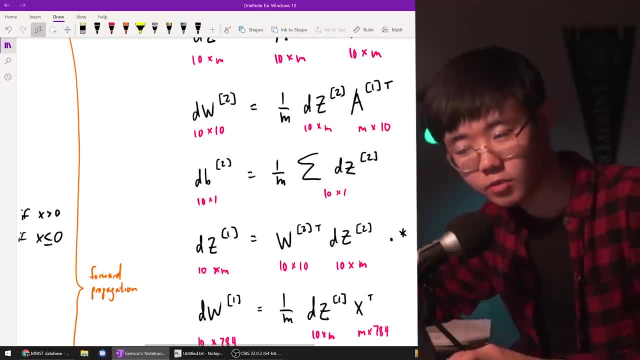 w and b contributed to that error. So we can find this variable dw2, that is the derivative of the loss function with respect to the weights in layer two, db2,. this one is really easy to understand. What this literally is is an average of the absolute error, right, Literally just the. 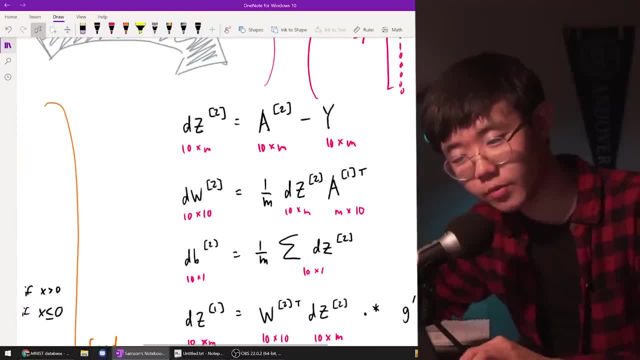 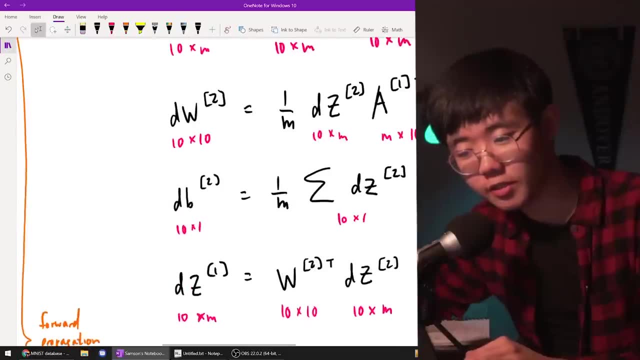 error, how much the output was off by. That's for the second layer. right, We're going to find out how much the second layer was off by from the prediction And then we find out correspondingly, how much we should nudge our weights and our biases for this layer. Now we'll 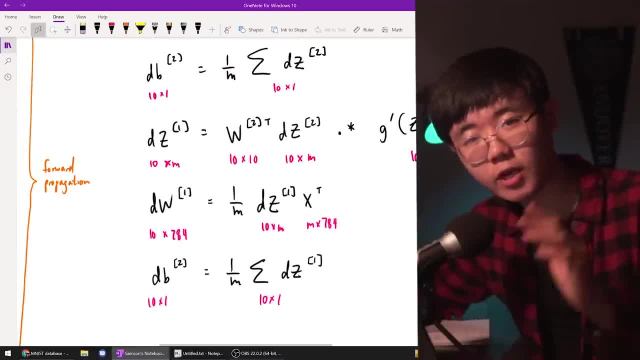 do the same thing for the first hidden layer. We're going to find dz1, right, How much that hidden layer was off by. And here there's a- there's a fancy bit of math here. That's the intuition is kind of that. it's just doing propagation in reverse, right Here you see this. 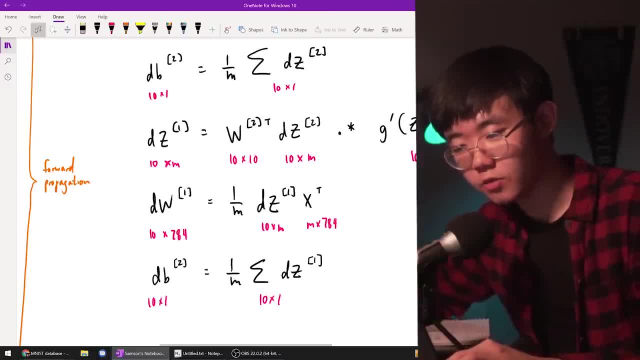 this weight for the second term, transposed times dz2, right, We're taking the error from that second layer and applying the weights to it in reverse to get to the errors for the first layer. And we're also taking this, this G prime, here. that's the derivative of the activation function. 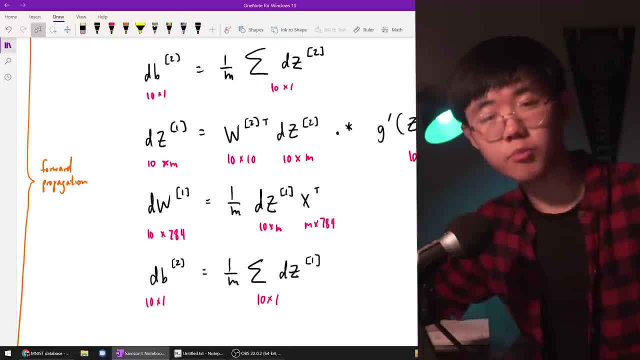 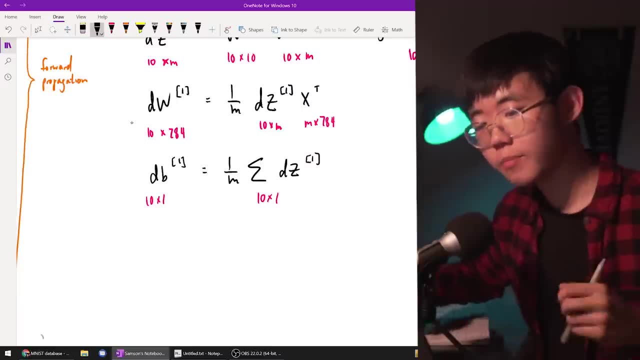 because we have to undo the activation function to get the proper error for the first layer. And then we do the same thing as we did before, to calculate how much w1 and b1 contributed to the error in the first layer, And that's how much we're going to nudge them by. So yeah, so after. 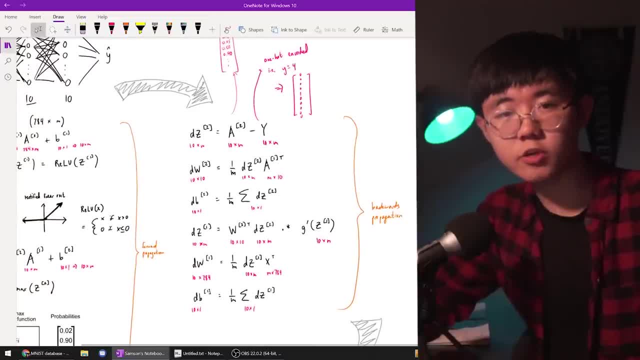 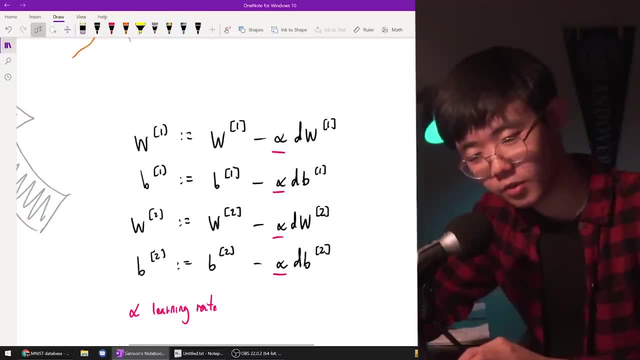 we do all this fancy calculation and figure out how much each one of these errors are. we're going to take the weight term. each bias term contributed to the error. we update our parameters accordingly. So this is a set of pretty simple equations. right: w1 is equal to w1 minus alpha. 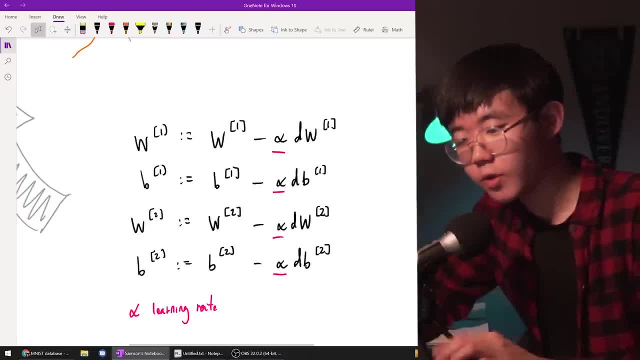 some learning rate: alpha times dw1.. Similarly, b1 is b1 minus alpha times db1.. w2 is w2 minus alpha times dw2.. And b2 is b2 minus alpha times db2.. Alpha is what's called a hyperparameter. It's not. 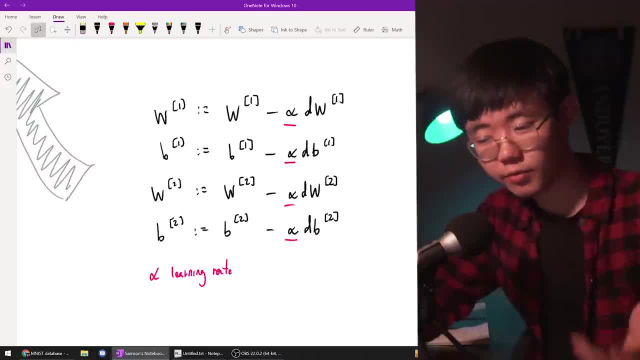 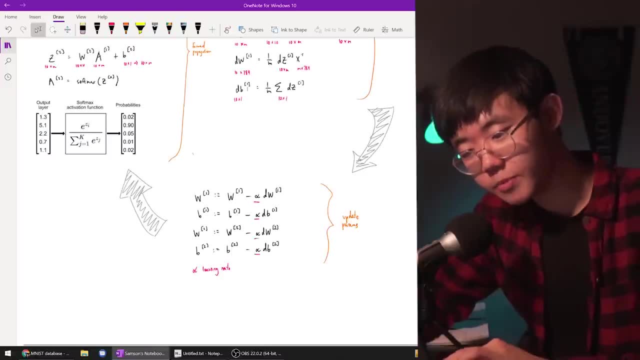 trained by the model The, the. when you run this cycle, when you run gradient, gradient, gradient descent, the learning rate is a parameter that you set, not that gradient descent set. So once we've updated it, we run through the whole thing again, We go through forward prop, we make a new. 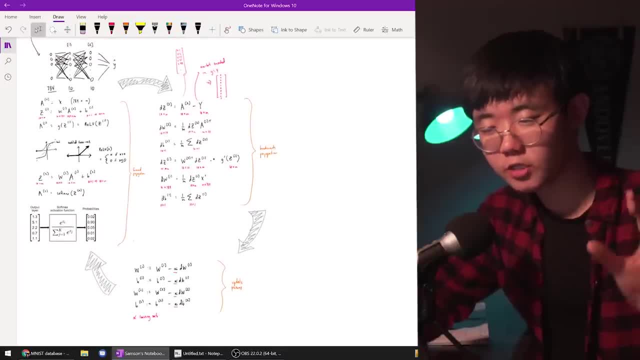 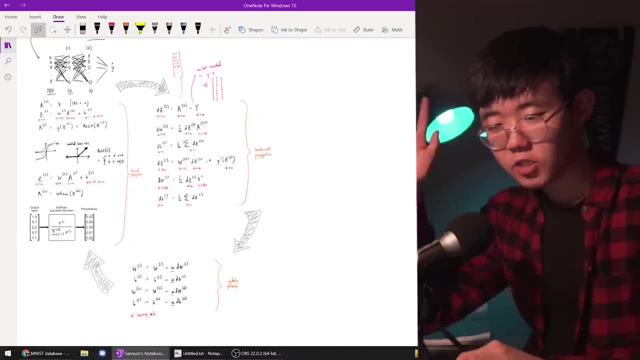 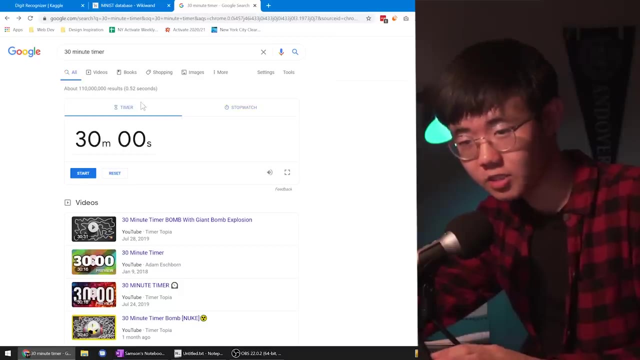 round of predictions. we are changing our parameters, tweaking them so that the prediction is ever closer to what the actual correct answer should be. That's math. Now let's get to coding it up. I'm going to attempt to do it in the next 30 minutes. Bye. 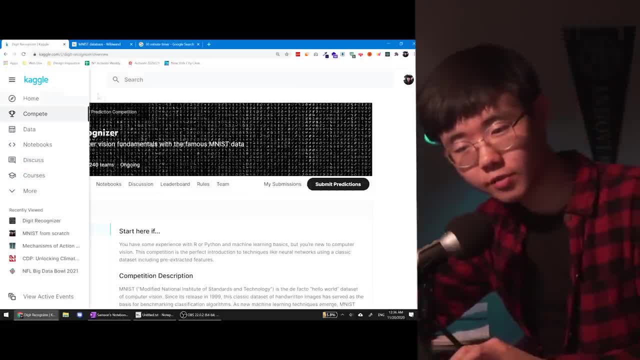 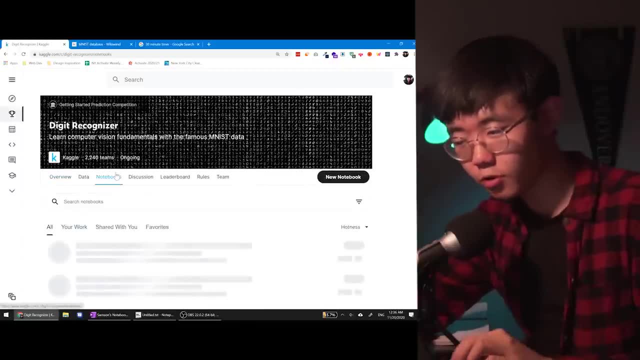 We're going to be doing this on a site called Kaggle Kaggle. is this really great site that makes it really easy to access data sets and have notebooks, have Python notebooks, Jupyter notebooks. So our digit recognizer data set is already nicely configured here. 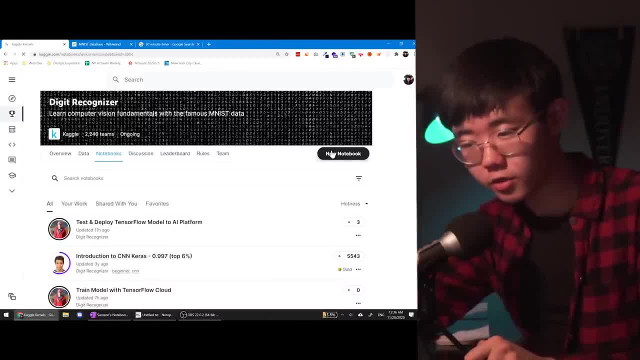 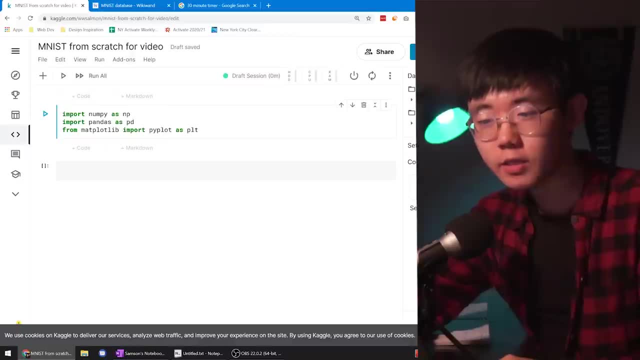 And all we have to do is hit new notebook and we will be taken into a kernel. Here we are: we have a notebook And let's just rename it real quick. So the first thing that we're going to do is import our package. So NumPy is for linear alphabets, for, like, working with matrices And 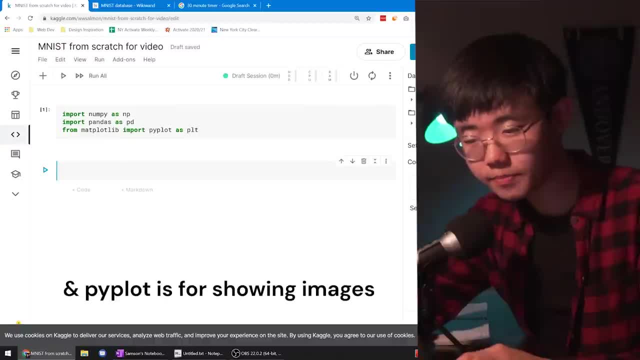 NumPy is just for reading the data. We're not going to use it much, So import. Next, let's import the data. So we're going to use pandas for this, So data is going to be equal to pandasread csv. I'm going to specify the file path So you can see how Kaggle makes it super easy to access. 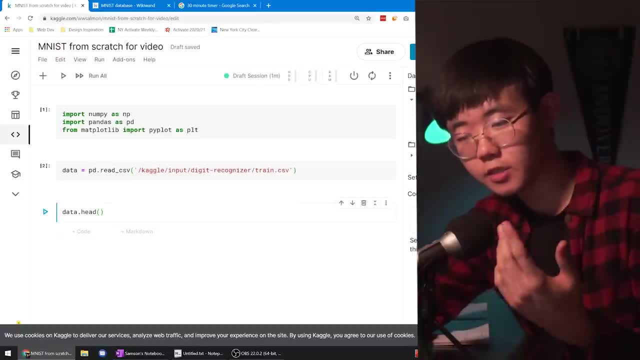 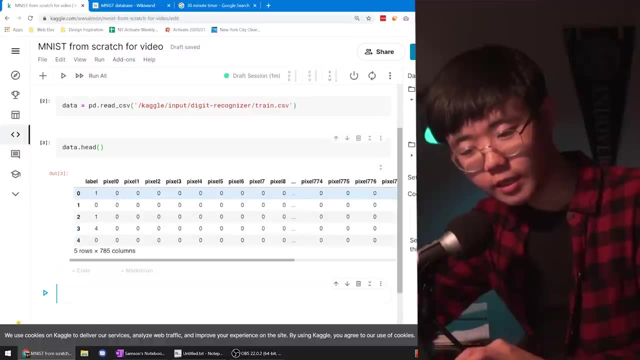 the data here Because it's pandas. it loads it in as a pandas data frame. We can call head on it and get a little preview of what's up here. Each row corresponds to one training example. They have a label and they also have all these pixel values for. 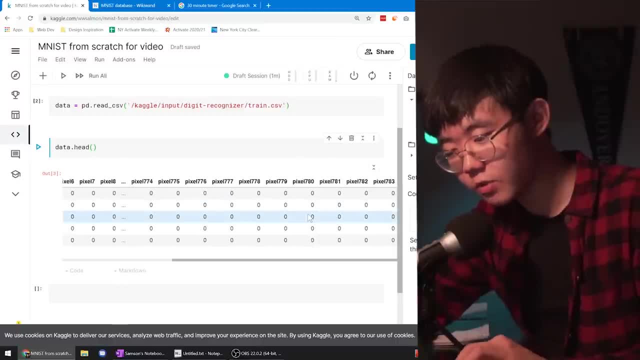 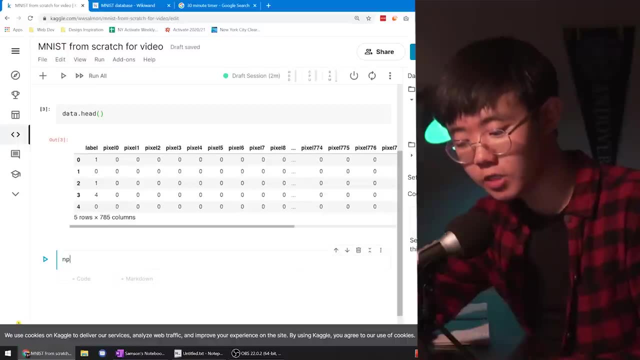 each example, We have pixel zero all the way to pixel 783.. So, inclusive, that is 784 pixels. we actually don't want to be working with a pandas data frame. we want to be working with NumPy arrays so that we can manipulate them and do fancy linear algebra with them. So we are going. 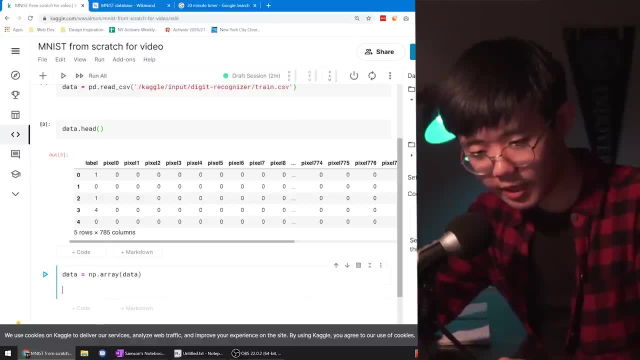 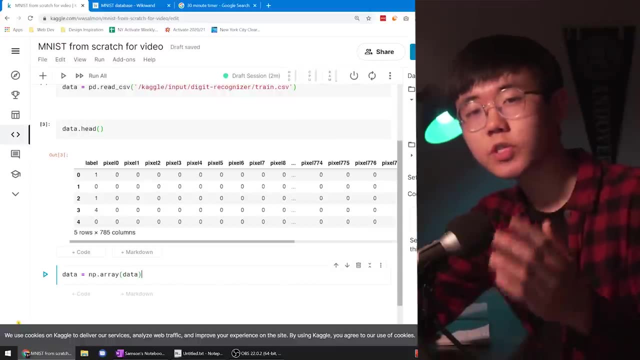 to say that data is equal to MP array of data. And then we are going to split up our data into dev and training sets. there's always a risk of overfitting right. there's a risk that your model is going to figure out exactly how to do it. So we're going to say that data is equal to. 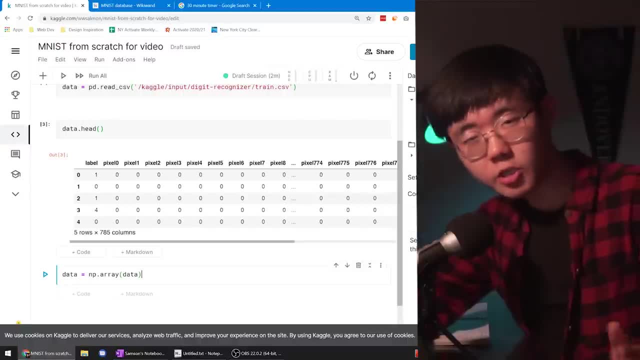 mp, and then that data is going to be how to make exactly the right predictions for your training data, but not generalize to the data that you actually want to be generalizing to. so you set aside a chunk of data that you don't train on, And that's your dev or your cross validation data. 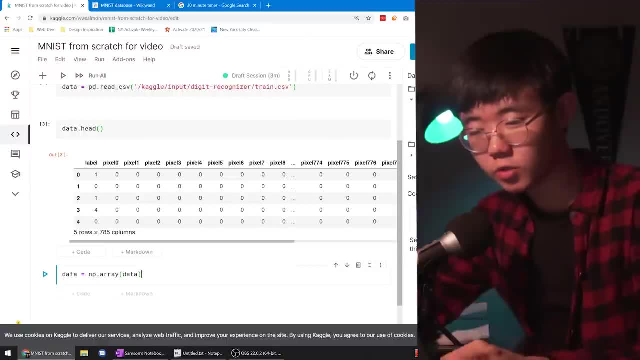 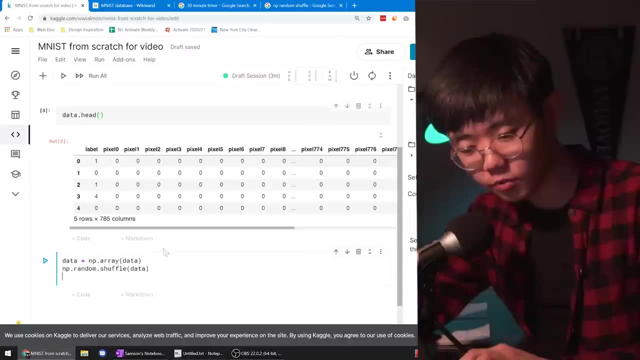 And that way you can test your hyper parameters on that data, you can test your performance on that data. you eliminate the risk of overfitting to your actual training data. we're going to shuffle our data, So hopefully it's just Mp dot, random dot shuffle. okay, Hopefully I'm not going crazy. 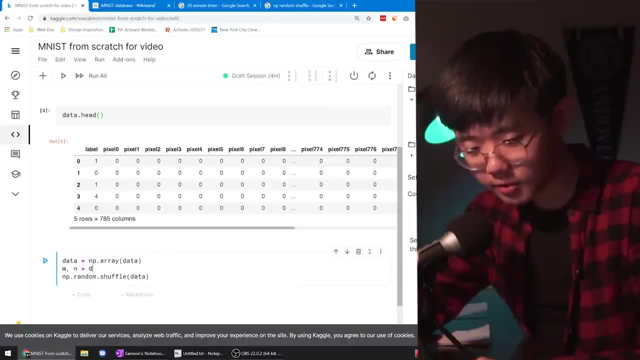 here. So m and n is going to be called datashape. So m is just the amount of rows, right? That's the amount of examples that we have, And n is not quite the amount of features. It's the amount of features plus one. 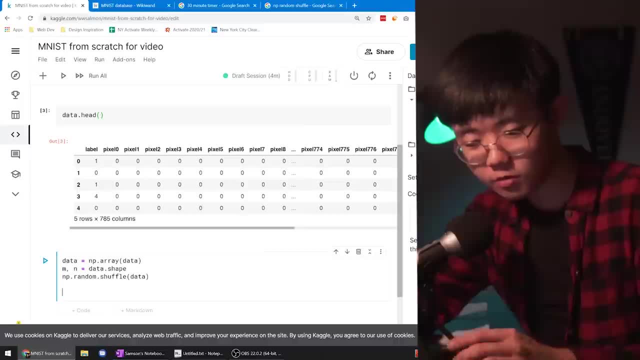 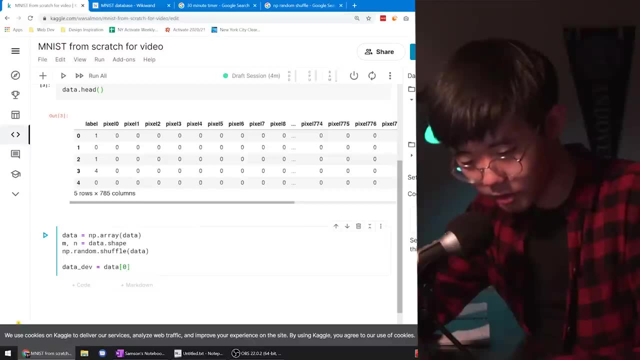 because we have this label column, but it'll be helpful to have that. So there we go, And now we're going to go. datadev is going to be equal to data from zero to 1,000.. Okay, the first 1,000 examples. 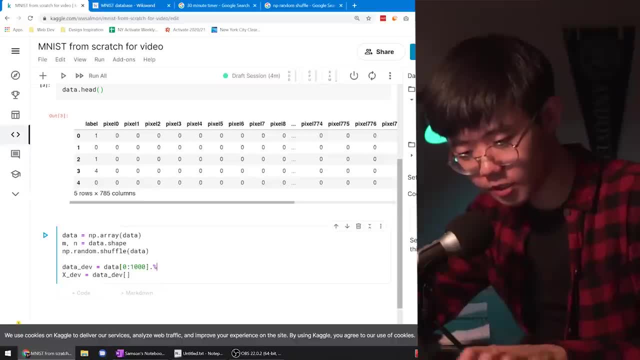 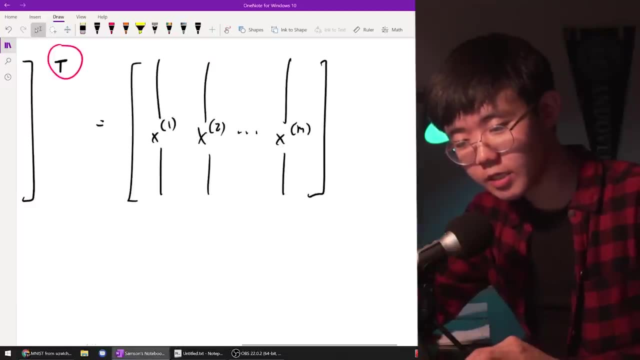 and then I want all of it. So I'm going to go with that. Okay, let's transpose this as well. Okay, so we're going to transpose it. So, if you remember, that's the thing where we flip it, so that each column is a example rather than each row. 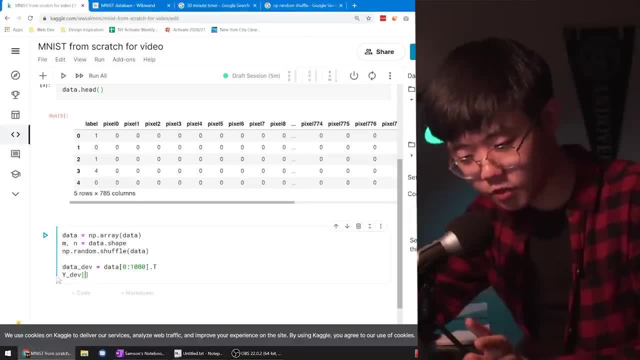 And that just makes it easier here. Y dev, if you remember, is now going to be the first row, right, It's going to be super convenient. Y dev- damn, what am I doing? Datadev zero and x dev is going to be datadev one to n. 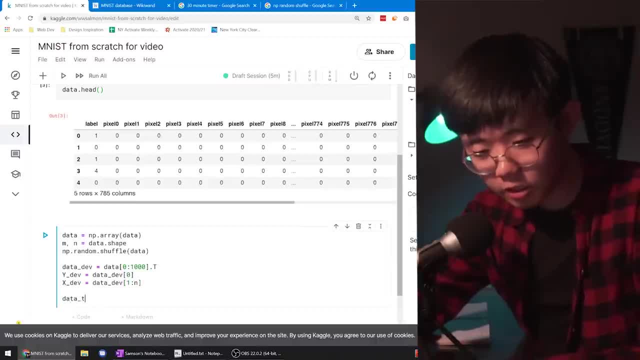 Remember that That's our n coming in handy here, And then our data train. this is the data we're actually going to be training on. It's going to be zero, sorry, 1,000 to m. So all the rest of it, transpose it again. 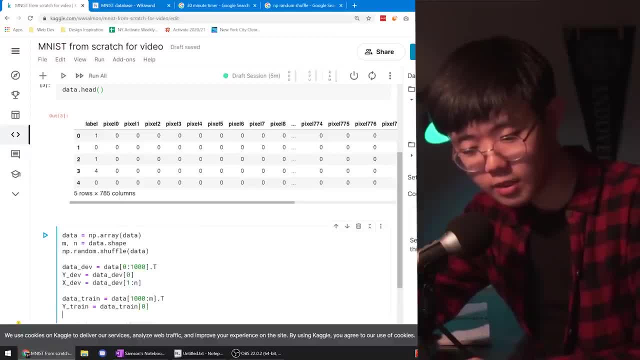 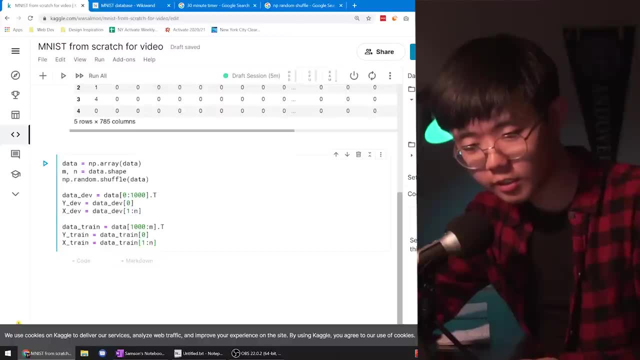 Y train is going to be equal to data train at zero, And then x train is data train from one to n- Beautiful. So this should be all of our data loaded in. Let's run that and take a look at, for example, y train. okay, 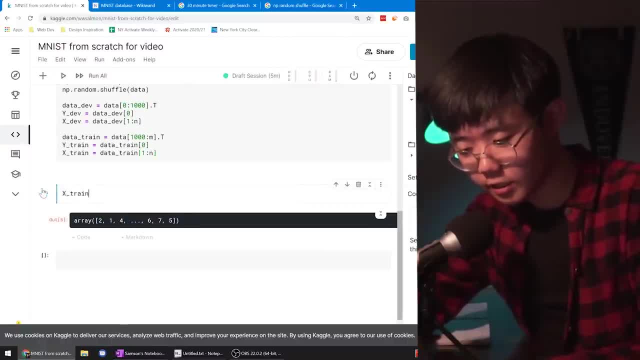 Y train. look at that. So we have an array of all of our labels. And then let's take a look at x train zero. Let's look at the shape. It's not super helpful. Look at that. Let's look at the first row. 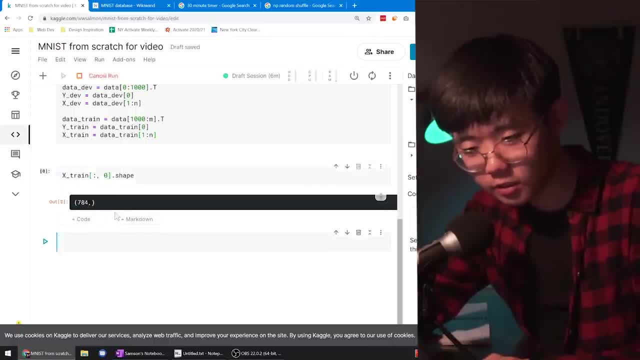 So that's actually not what I want. I believe I want this. There we go. So there we go. That's our first column, And it has 784 pixels in it. That's exactly what we want. So, okay, now we have our data. 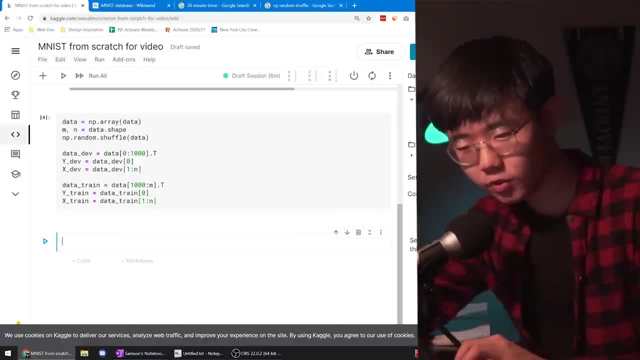 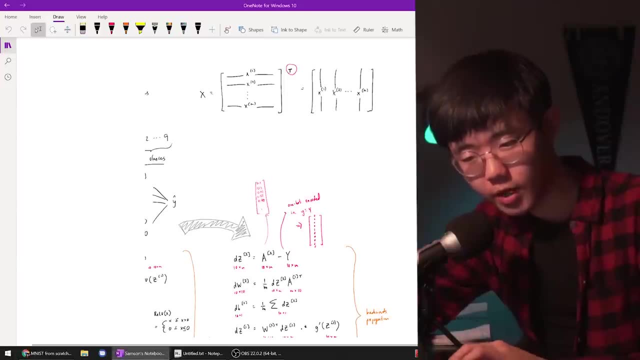 Now we can start just bashing out code for the actual neural network part. Let's see how much time we spent. Okay, seven minutes. We'll move fast. We'll move fast. The first thing we're going to do is initialize all of our parameters. 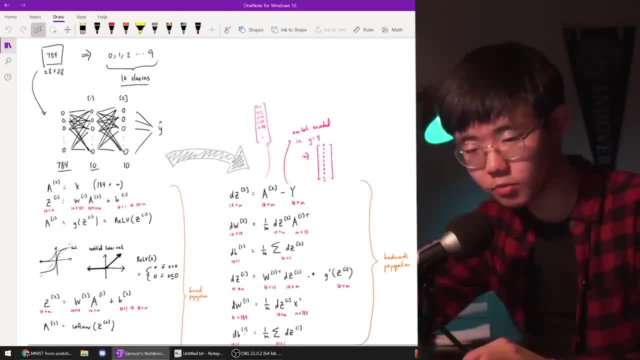 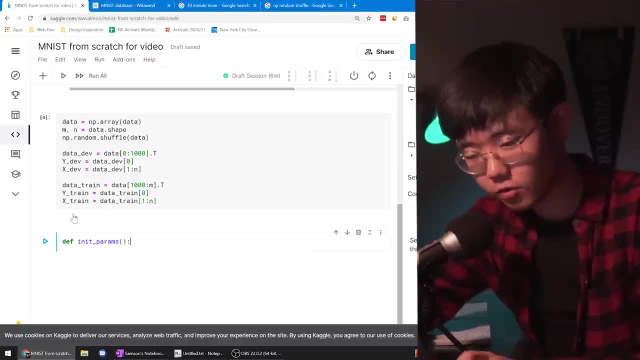 We need a starting w1., b1,, w2,, b2, right, And we have all of the dimensions for them here. So we're going to go def init params And this takes no arguments. It doesn't need any arguments for that function because it's creating. 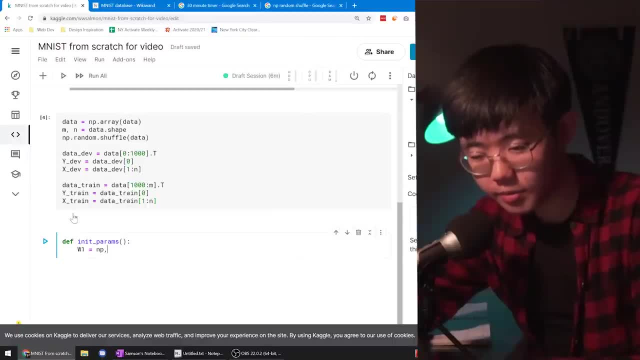 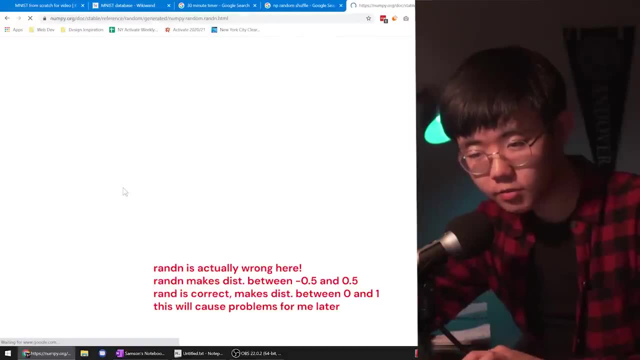 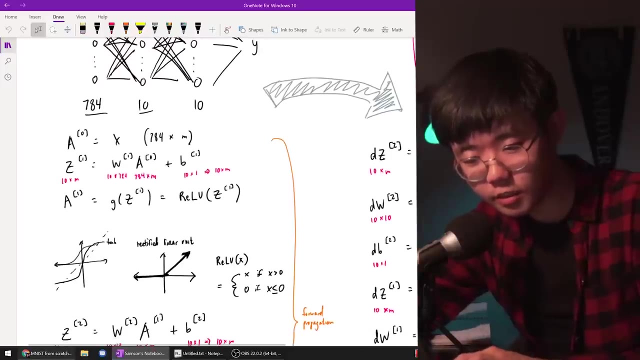 a complete from scratch. w1 is mprandom And I think is it that mprandom rand? I believe it's rand n. okay, And our first, and we want the dimensions of this array to be, w1 is going to be 10 by 784.. 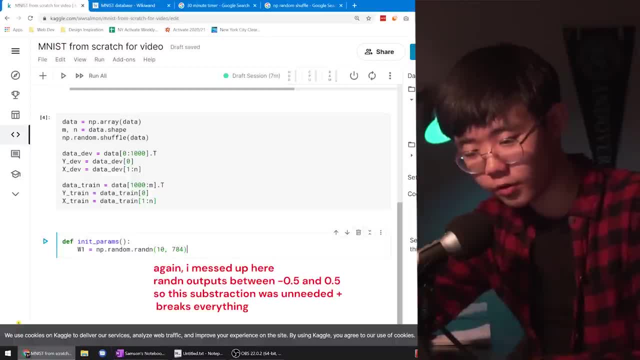 This is going to generate random values between 0 and 1 for each element of this array. So we're actually subtract 0.5 from that to get it between negative 0.5 and 0.5.. b1 is going to be mprandomrandom. 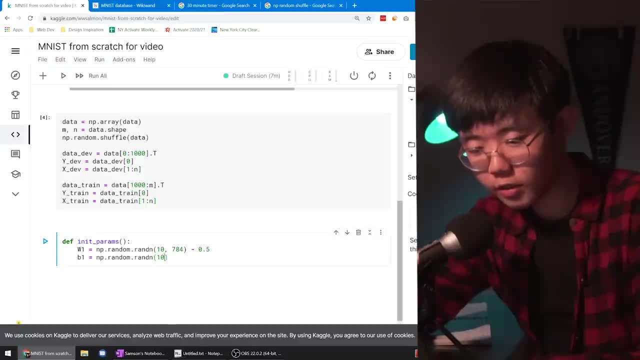 The dimensions here are going to be 10 by 1.. And again we're going to subtract 0.5 from that, And then same exact thing for w2, okay, So w2 is going to be 10 by 10.. 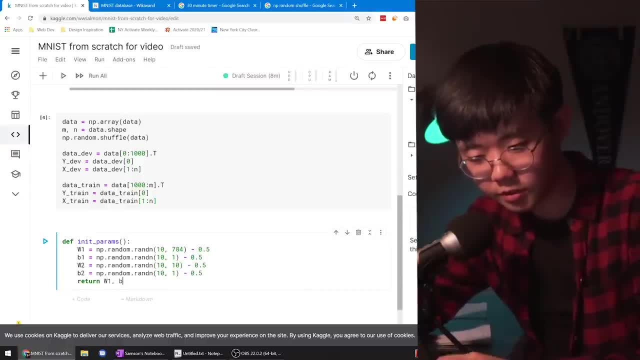 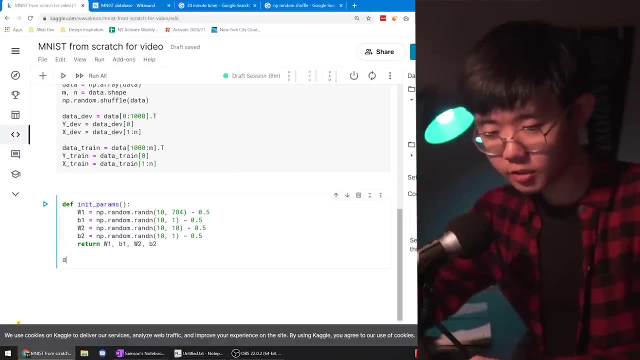 And b2 is going to be that, And then we're going to return all these values. okay, After we initialize the params, we are basically ready to go into forward propagation. So we're going to go def forward prop And this is going to take w1, b1, w2.. 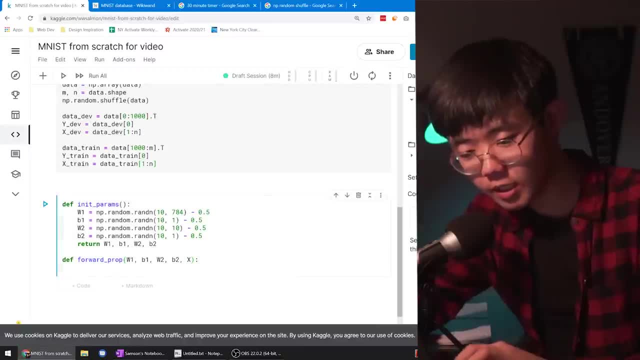 b2 is arguments, And also x. we're also going to need x. So first we're going to calculate. let's calculate z1.. Okay, So z1 is going to be equal to w1 dot. So remember w1 is a numpy array. 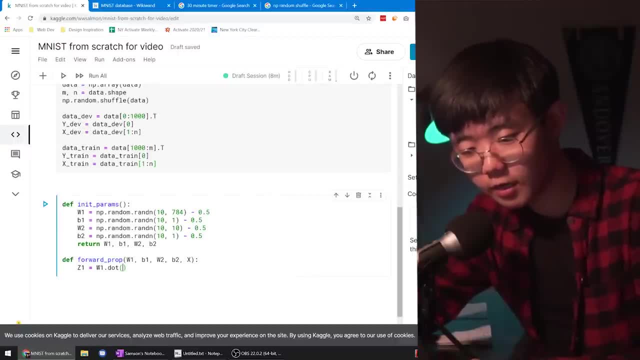 So we can do matrix operations using this: dot, dot, dot x. okay, Plus b1.. Now a1 is going to be equal to rel u of z1.. But rel u is not defined, So let's define rel u here: Rel u of z. 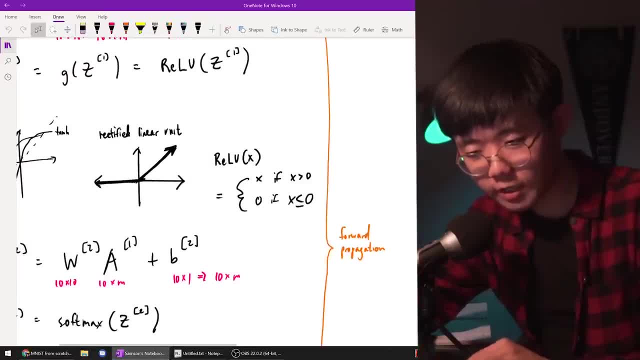 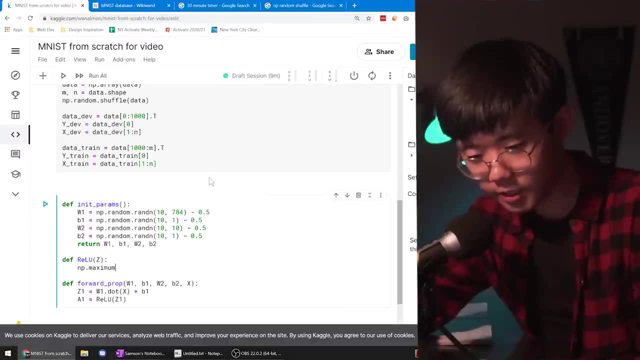 And remember, rel u is just this linear function, Right here. right, It's going to be x if x is greater than zero and zero if x is less than or equal to zero. There's a pretty elegant way to do that. So that's np dot maximum. 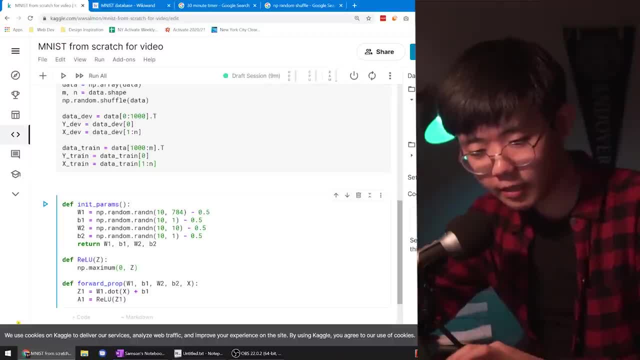 And we're going to take the max of zero and z, And this is element wise. So when we take maximum like this, what it's doing is it's going through each element in z. If it's greater than zero, it's just going to return z right. 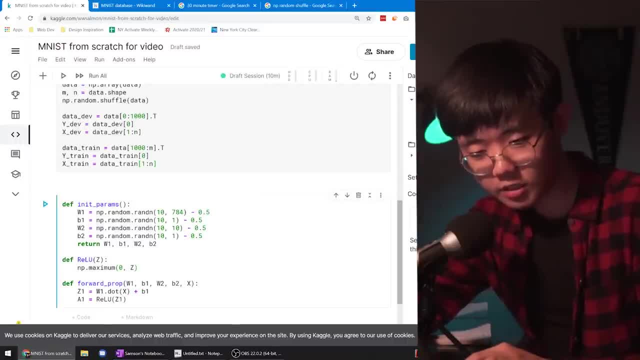 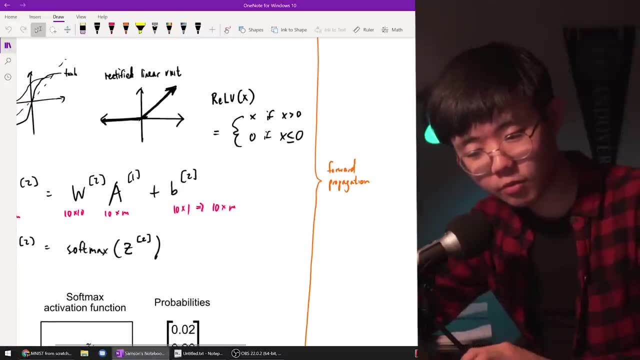 But if it's less than zero, it's just going to return zero. So this is exactly what we want. We'll return that. So a1 is going to equal So rel u of z1.. That's exactly what we want. 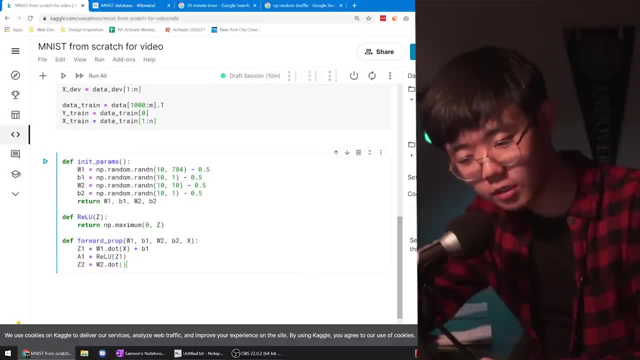 Great, And now we'll do z2.. z2 is going to be equal to w2. dot a1 now plus b2. And then a2 is going to be equal to softmax of a1. And again, we're going to need to define softmax now. 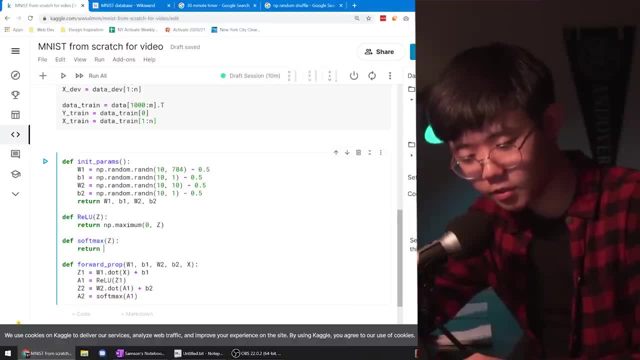 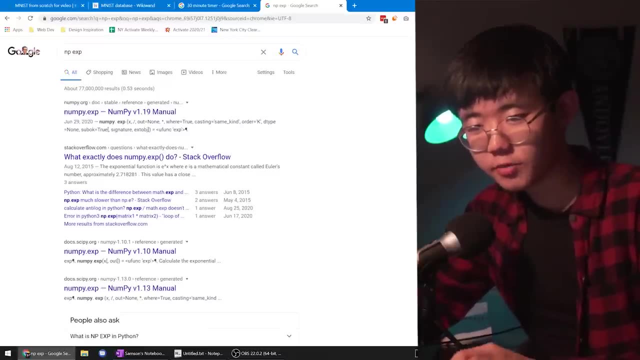 Softmax of z, And we're going to return Here it's going to be. We're going to reference this formula right here And what we can actually do is np, dot, exp, And remember that's just e to the x, right. 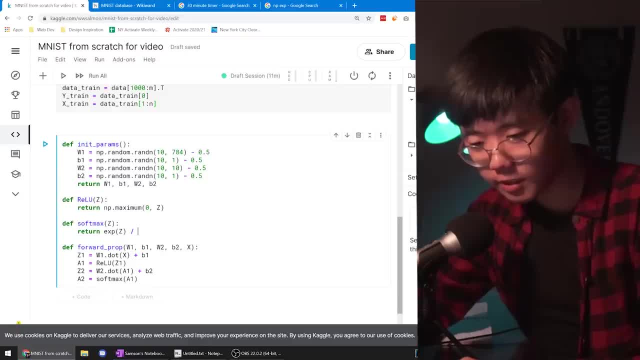 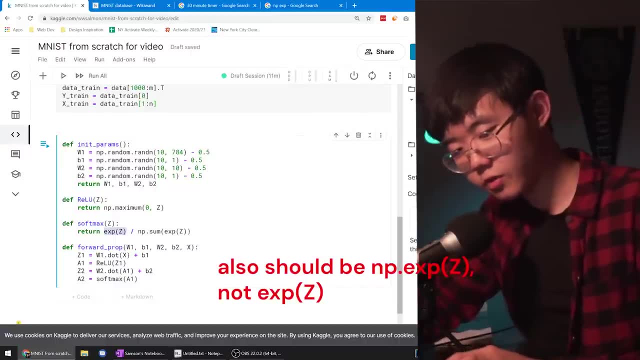 And we're doing that to each element of the array. So we're going to do this: Divided by np dot sum of exp across z. First it just applies like e to the z, to every single value, And then np dot sum is going to sum up through each column. 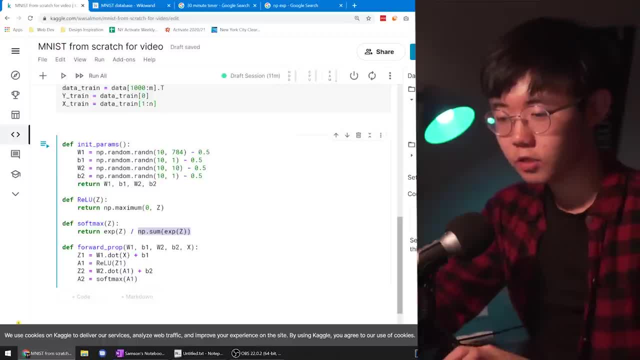 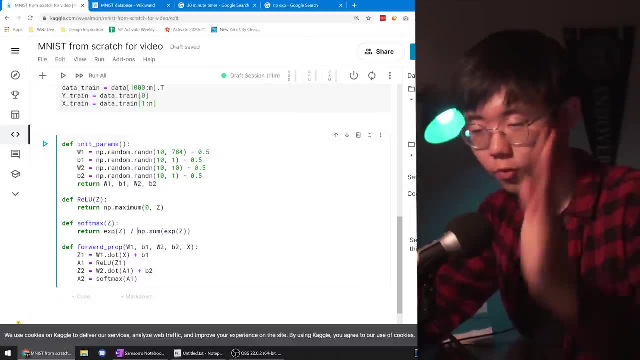 So it preserves the amount of columns and then collapses the amount of rows to just one to get this sum right. And that's exactly what we want. We want the sum for each column across all of the rows in that column, And we want to divide each element by. 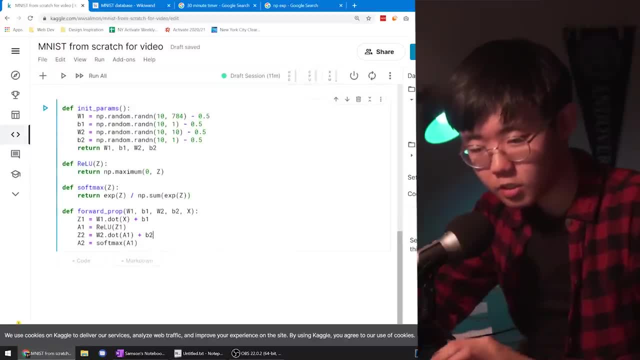 And that's going to give us the probability that we want. So there we go. That's forward prop. Forward prop is done. Now in back prop we are going to take in. Let's just take in all of these, Okay. 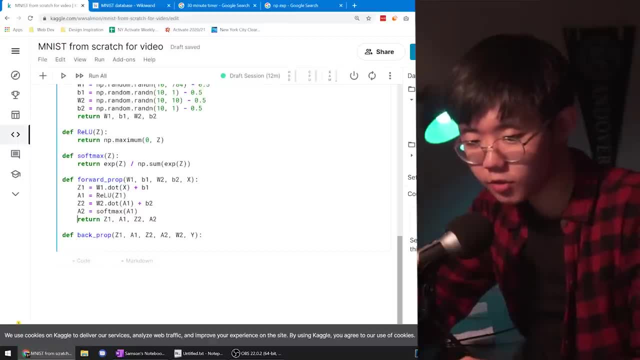 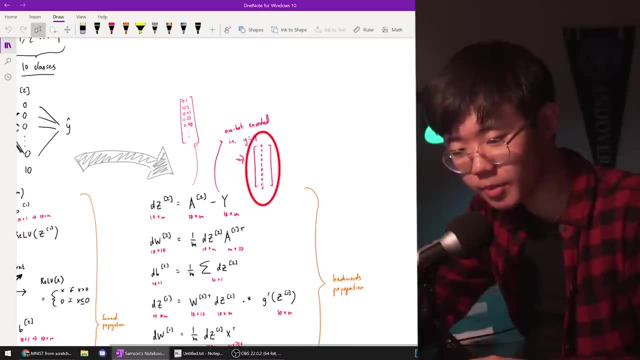 Beautiful. So the first thing that we're going to do is we actually need to do one thing to y. We need to one hot encode y. We need to take these labels and turn it into this matrix thing here, remember. So, oops. 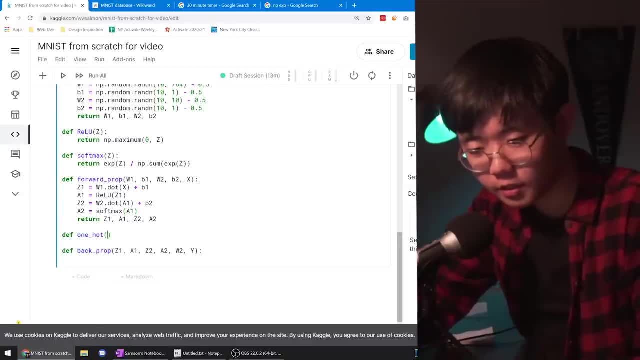 We are going to define a function: one hot, Okay. Okay, Take in y. And here I've actually cheated a little bit And I've taken one hot from when I did this previously. What this is doing is: first it creates this new matrix- one hot, y right. 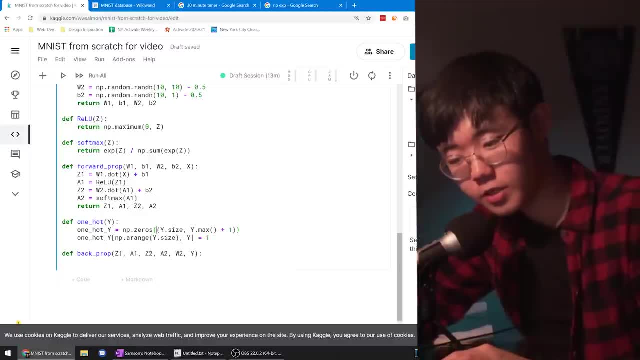 Which is just mpzeros. It's an array, a matrix of zeros And this is a tuple of its size, right? So ysize is just the length of size. So this is m right. This is how many examples there are. 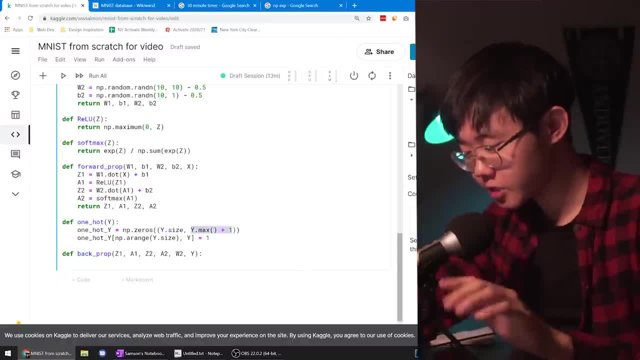 And then ymax plus one. It assumes that the classes are, you know, zero through nine, right? So the max is going to be nine, And then we add one to that and we get 10, which is exactly how many output classes we want. 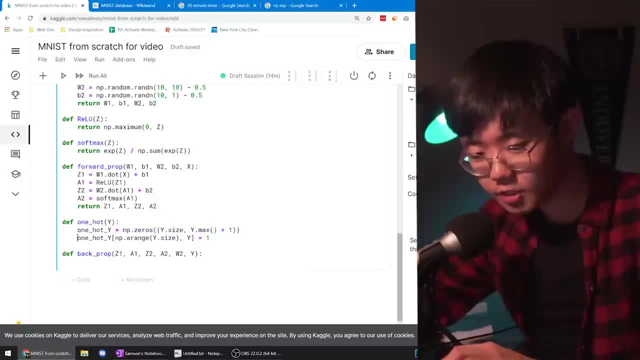 So this creates the correctly sized matrix for us, And this is a really cool thing. You're indexing through one hot y using arrays right, mparange, ysize. This is going to create an array, right? That's just the range from zero to m, right. 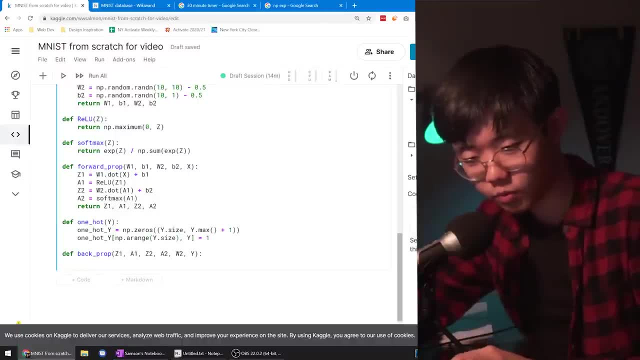 To the number of training examples, And that specifies what row this is accessing. And then y remember, is our whole thing of labels right? This is going to be like zero, one, four, one, seven. whatever. This is going to specify what column it accesses. 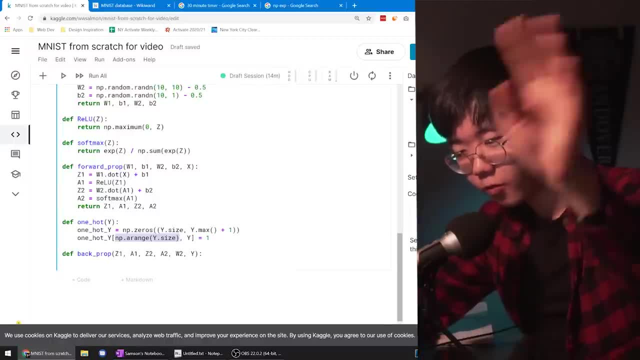 So what this is doing is it's just going through and it's saying: for each row, go to the column specified by the label in y and set it to one right. And that's beautiful. That's exactly what we want. That'll do the one hot encoding for us. 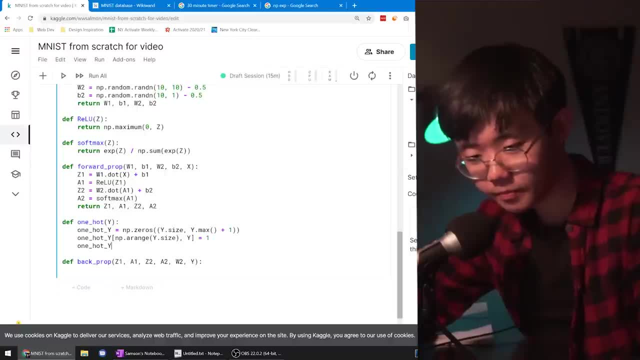 And then the one last thing we want to do is just flip this. okay, Hold on One hot yt and then we can return one hot y. And we want to flip it because right now, each row is an example And we want it the other way around. 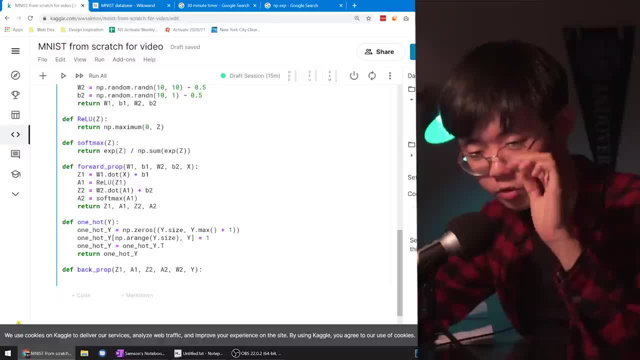 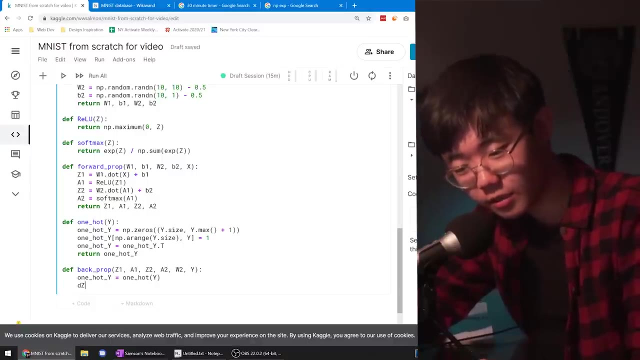 We want each column to be an example, So we'll transpose it and return it back here. So perfect, Now we're going to go. one hot y is equal to one hot of y, which you look at that. And dz, z2, okay, this is a new variable- is equal to a, to our predictions, minus one hot y. 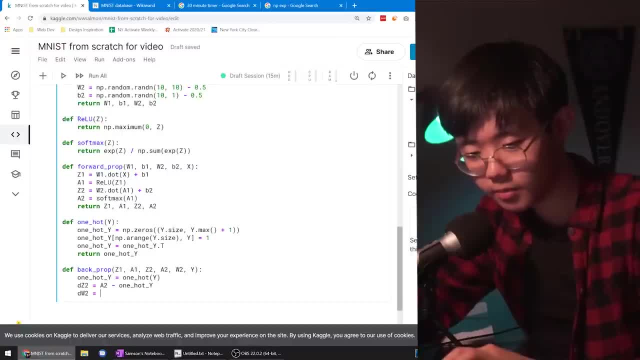 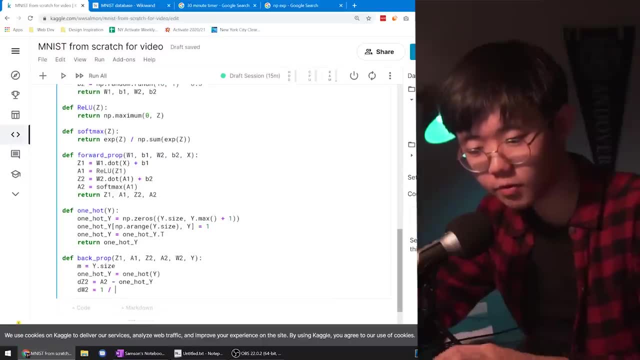 dw2 now is going to be equal to one over m. Okay, let's define m. m is going to be ysize, okay, just like we did before. One over m times dz, oops, dz2,. looks like this is a dz2.a1.t. 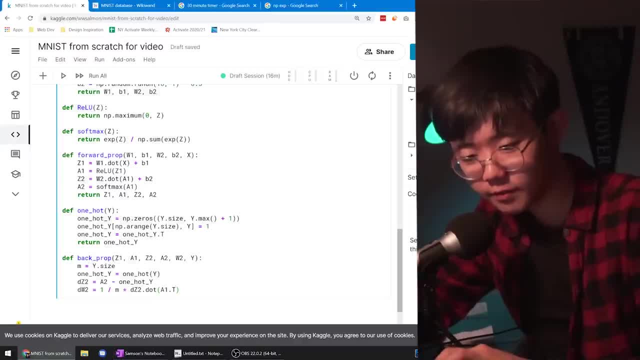 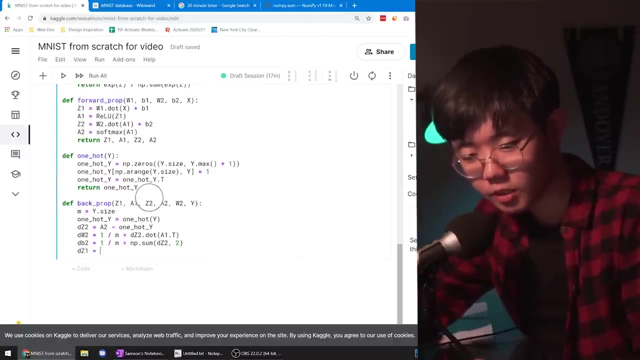 Yeah, I believe that's right. I believe that's right. Next, db2 is. db2 is just one over m times mpsum of dz2.. And then we want our dz1, which is going to be our fancy formula here. 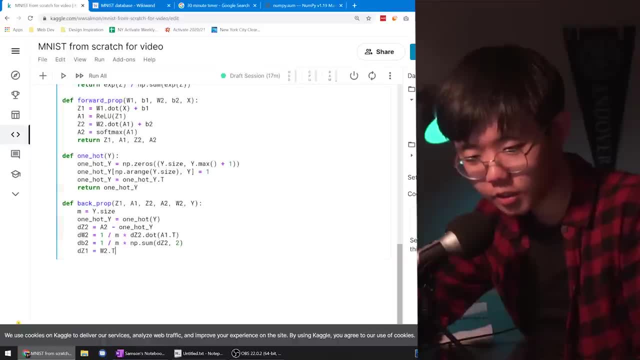 It's going to be w2.transpose dotted with dz2.. Okay, Okay, So this is kind of applying the weights in reverse, And now we're going to have to implement the derivative of the activation function in layer one. And the activation function in layer one, remember, was relu. 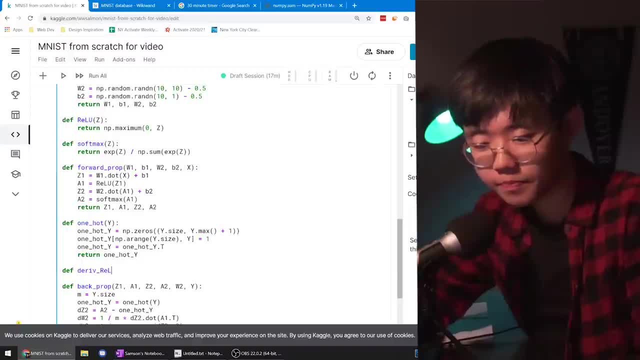 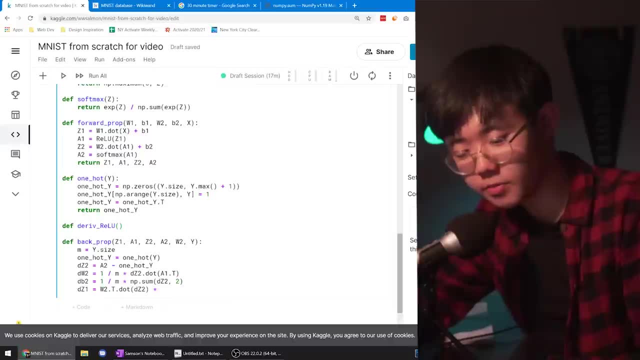 So we're going to implement the derivative of relu And that seems kind of fancy at first And I was freaked out when I was first seeing it. I was like how on earth am I supposed to do this? But it's actually really easy. 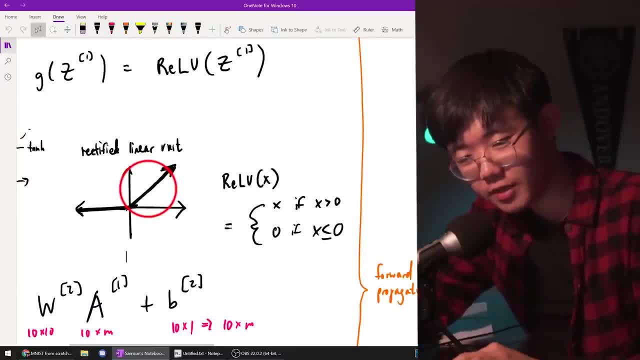 Just think about your calculus, right. What is the slope of this part here? It's one, right. It's just a. it's just a linear, linear thing. What's the slope of this part here? It's zero, right. 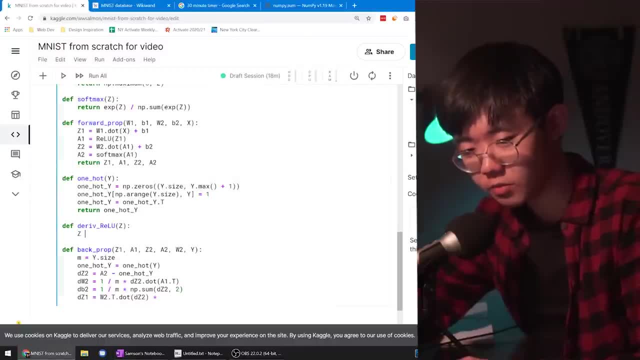 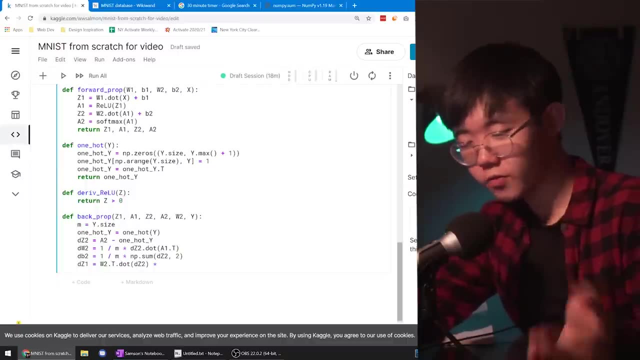 It's a flat line, So a really elegant way to do this is just return z is greater than zero. This works because when booleans are converted to numbers, true converts to one and false converts to zero. If one element in z is greater than zero, we're going to return one, and if otherwise, 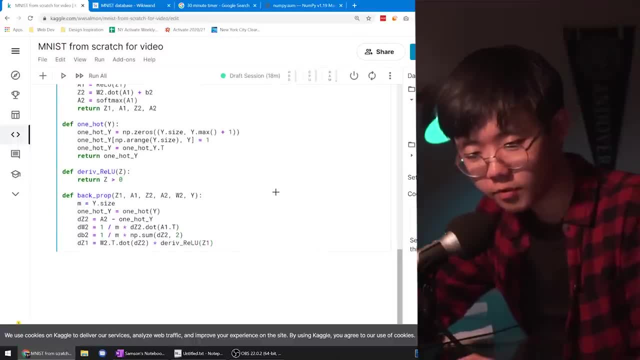 we're going to return zero, which is exactly the derivative that we want- Beautiful. And then now the same thing, as same thing as we did before. Okay, I believe it's. it's actually going to want x as well, because we're going to have xt. 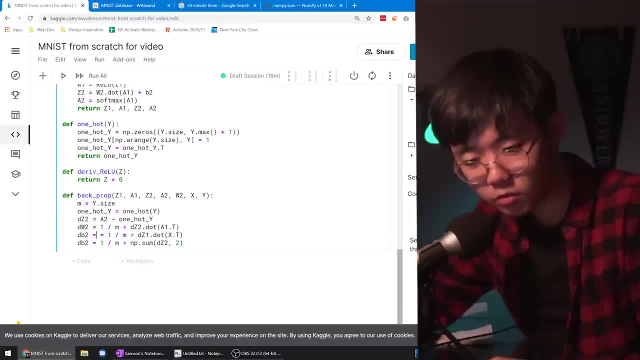 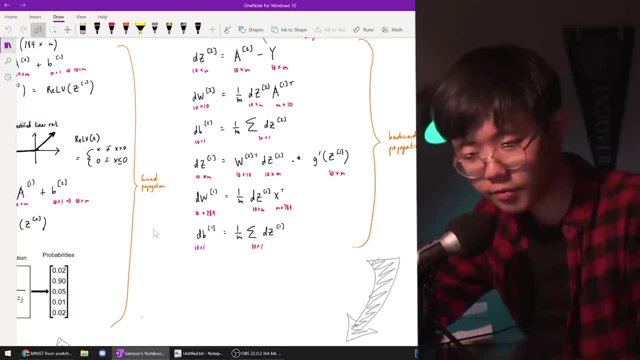 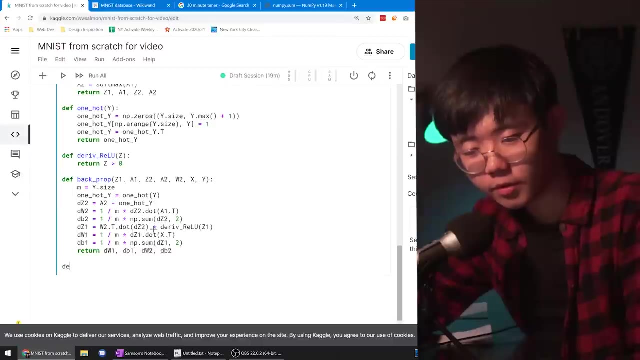 xt here, dz1,. oh, my goodness, that was not what I wanted to do. come on, There we go, And then from here we're going to return dw1,, db1,, dw2,, db2, and we're going to go def. 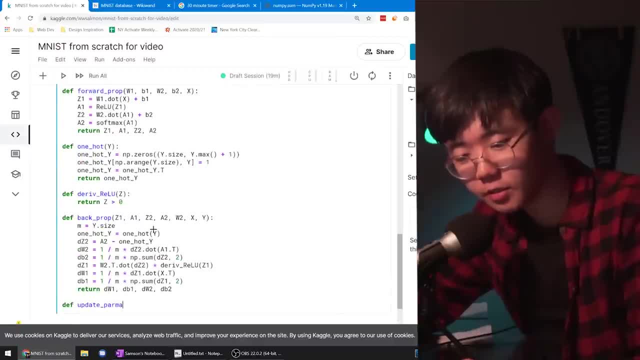 def. update params. now, All right, So update params. and we're going to take in here dw1,, db1,, dw2,, db2, and actually before that I'm just going to take in w1, b1,, w2, b2, and then alpha right, and we're 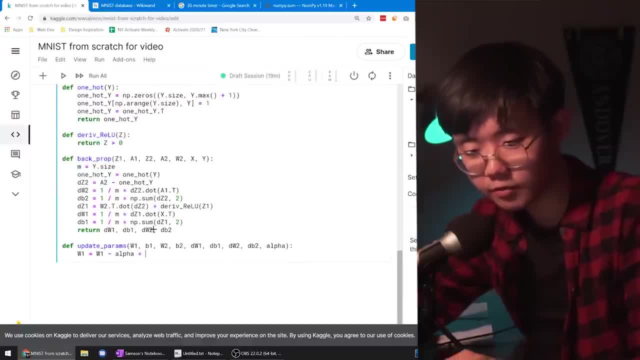 going to go: w1 is equal to w1.. This part's really straightforward: right times, alpha times, dw1 to b1 equals b1 minus alpha times db1.. And then we'll do the same thing here, Okay. Okay, So we'll do the same thing for 2, and then we're going to return our new w1,, b1, w2,. 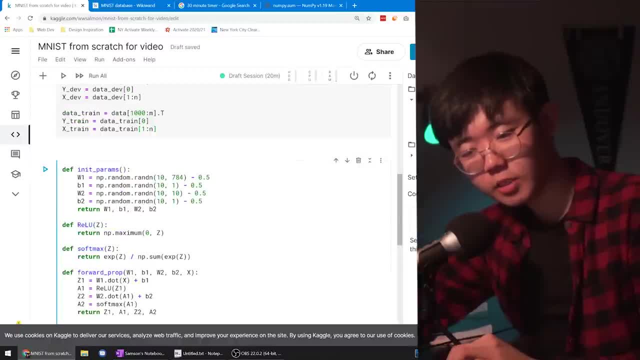 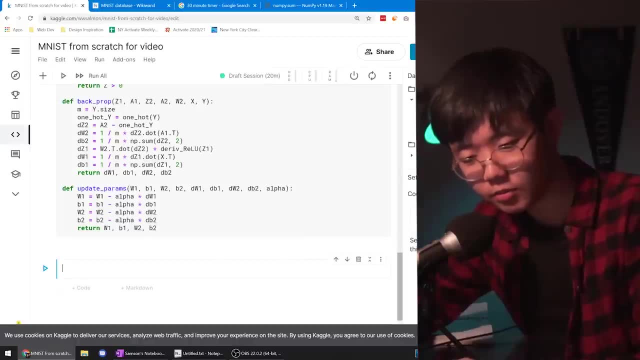 b2. Perfect. So in theory, if that's correctly implemented, that is all of the functions that we need for doing our gradient descent on our neural network: def gradient descent. That's what we're going to do now. We're going to take x and y first, because we need both of those, and then we're going. 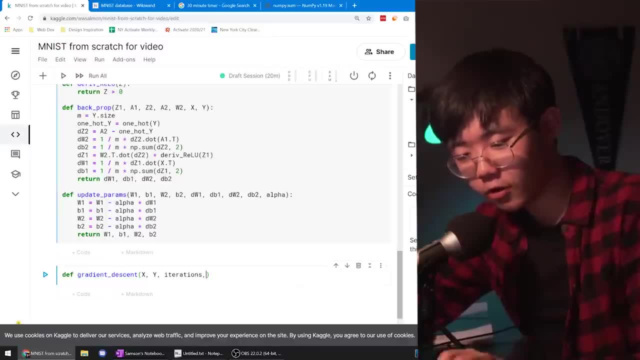 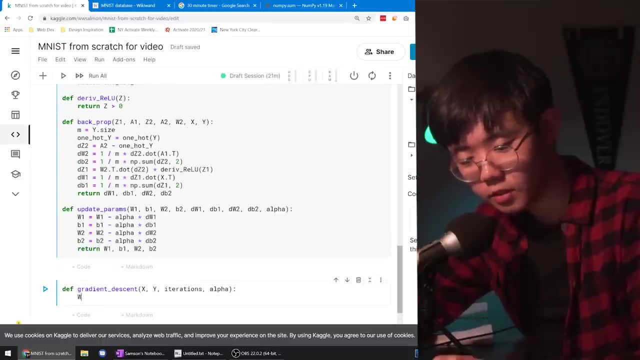 to take iterations alpha, and I believe that's all that we need. So first we're going to go w1, b1, alpha, Okay. Okay, W2, b2 is equal to init params. Okay, That's going to return us that. 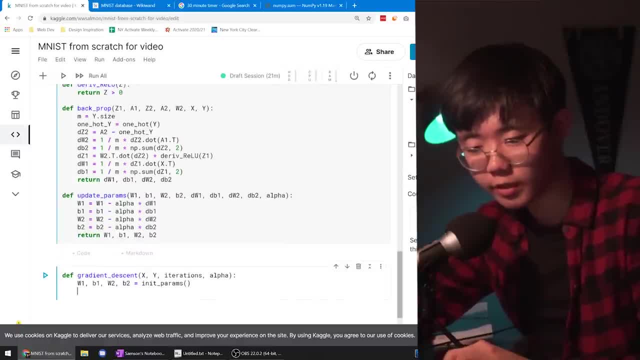 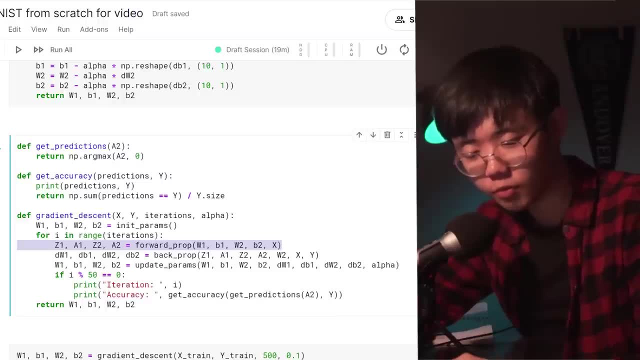 These are our initial values And now we're going to run that loop we were talking about right. So for i, in range iterations: first we're going to go forward prop right- z1, a1, z2, a2 equals forward prop- and we're going to pass in w1, b1, w2, b2.. 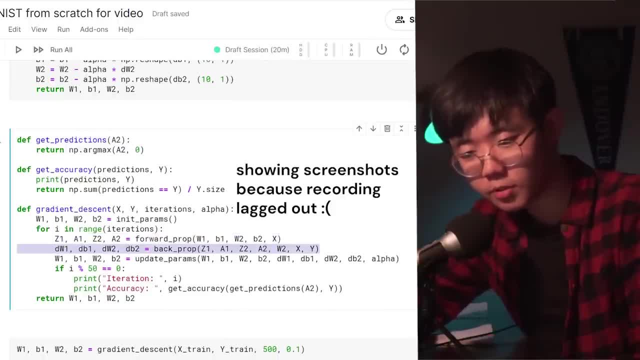 Next, we're going to get our wdw1, db1, dw2, db2.. Okay, And then, lastly, we're going to update our weights right when I say w1, b1,, w2, b2. 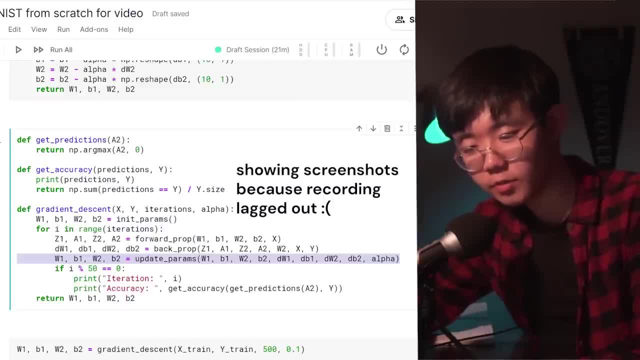 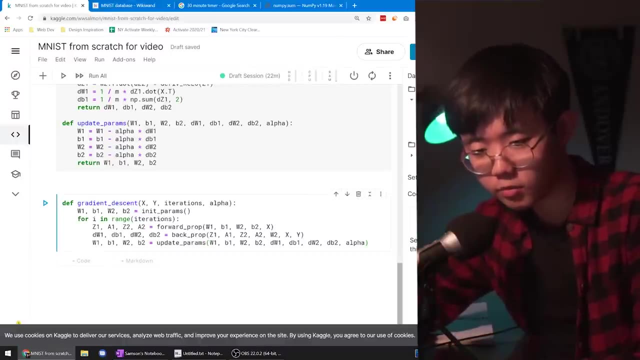 is now going to equal to update params w1, b1, w2, b2,, dw1, db1, dw2, db2, and alpha, And that's going to run a bunch of times and by the end of it it will return the params. 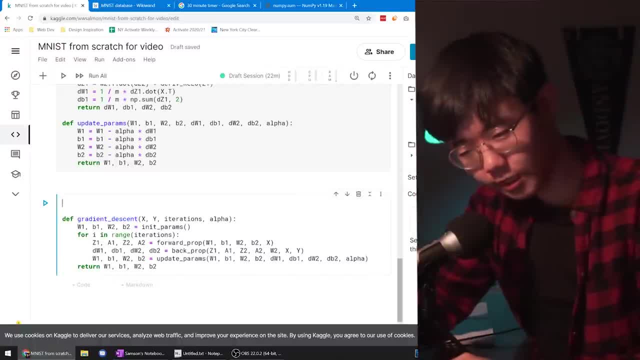 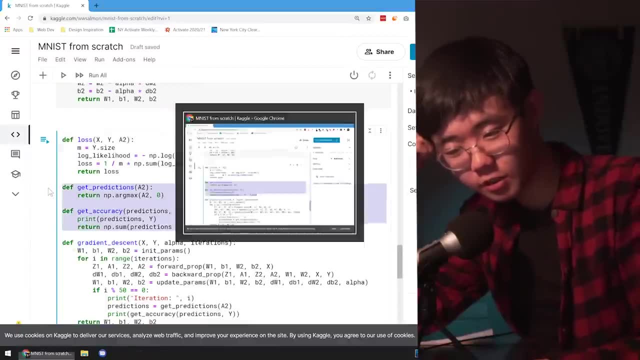 that we want. Okay, So we're going to do a few things, just so that we can actually see our progress. I'm going to cheat a bit and check the time that I did this last. We're just going to steal these two functions here, all right. 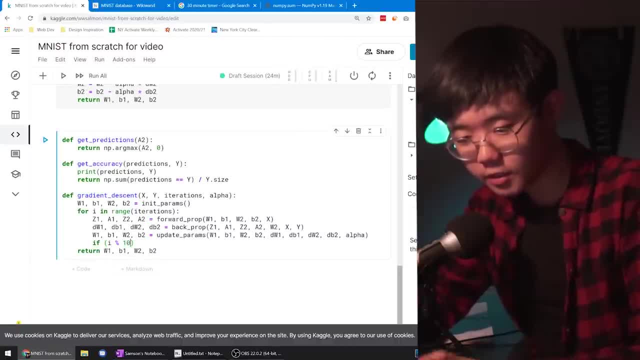 What we're going to do here is, if i mod 10 is equal to 0, so every tenth iteration we are going to print iteration and i and then print accuracy. Oops, This is going to be a little ugly. Get predictions a2.. 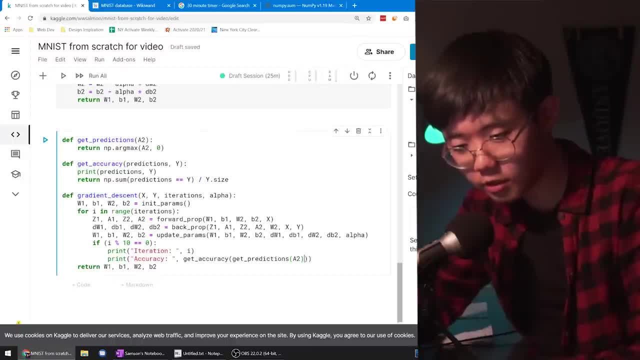 All right, So we're going to take our a2, which is our predictions from forward prop, and get predictions from those and then get accuracy on that and y Okay, And then it will return that. So let's run that. 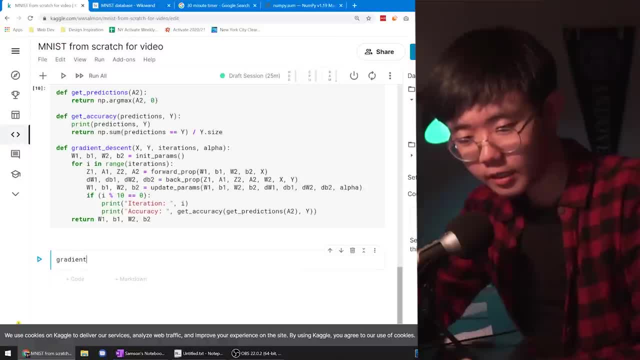 So all of those functions are defined now. Now let's run gradient descent and see what happens. And I'll take these parameters: w1, b1, w2, b2 is equal to 0.. Okay, So gradient descent, x, y iterations. oh, x, train, y, train. 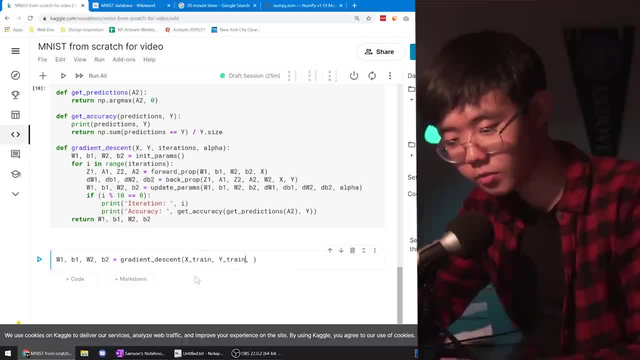 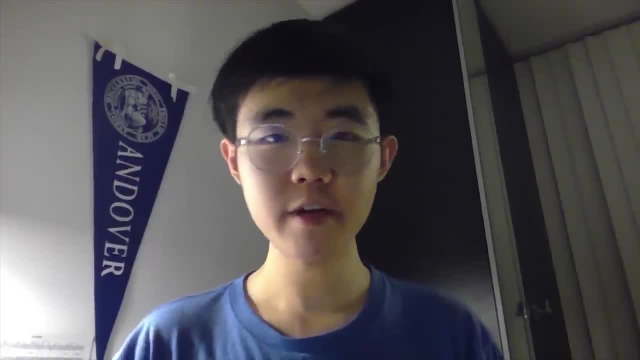 Now we're using the actual variables and we're going to go for, let's say, 100 iterations with a learning rate of 0.1.. Editing Samson here. So, because of those two errors early in the video, namely initializing weights and biases, 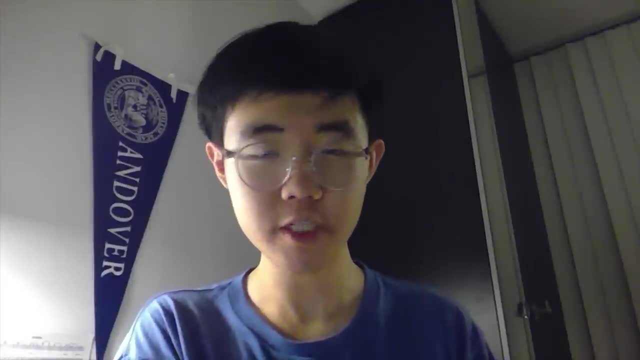 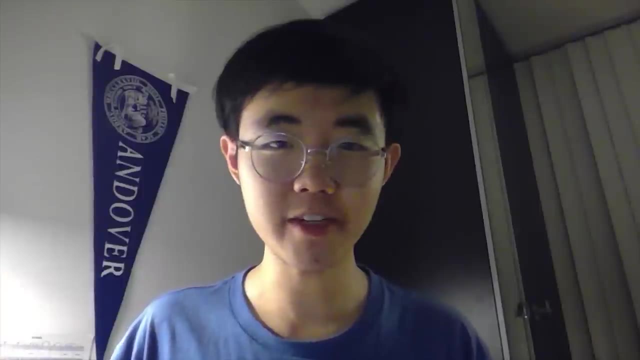 to all negative numbers and putting in an a1 where there should have been a z2, of course the model did not run well. It ended up with 10% accuracy, which is just random guessing, And I spent like an hour just debugging in the end just to change those two variables. 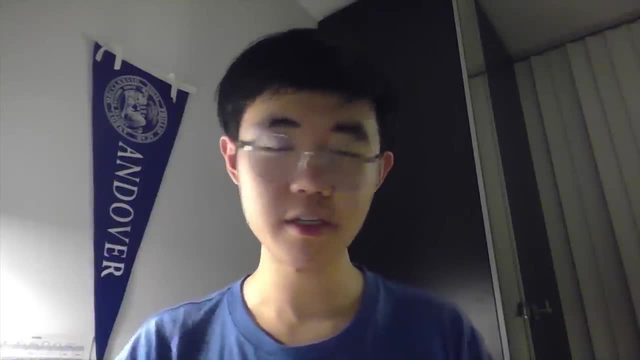 right. All the rest of the code is okay. I didn't change any of that. I'm just going to skip over all of that in editing and we're going to go straight to the end, straight to an hour later, when I figured out what was wrong and finally ran. 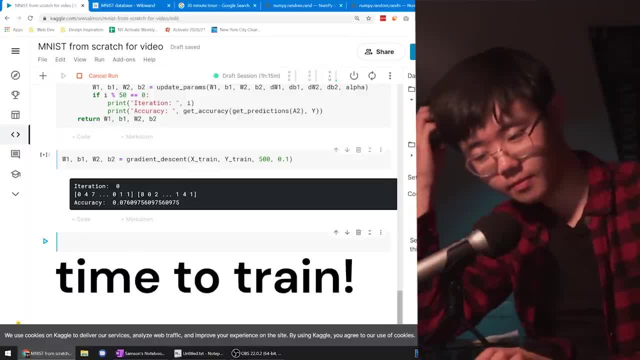 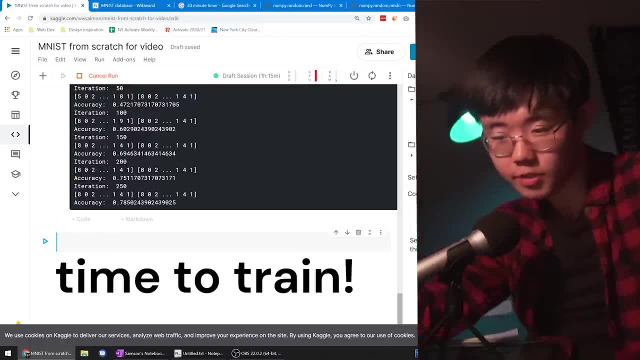 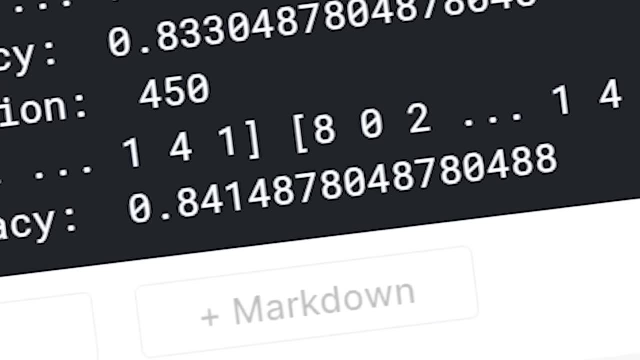 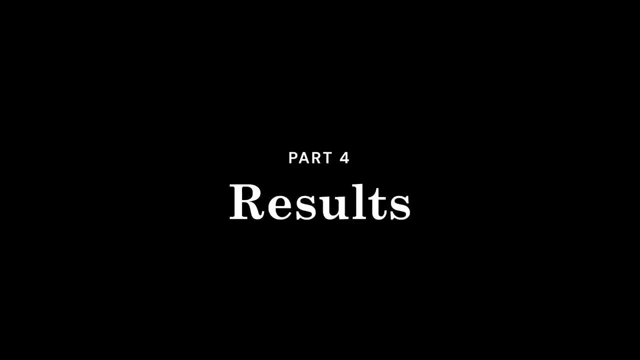 the model And let's go here. But look at that: 75% accuracy, 78% at iteration 250.. Okay, 84% accuracy on training data is what we got, So there's definitely a lot of room left for improvement. 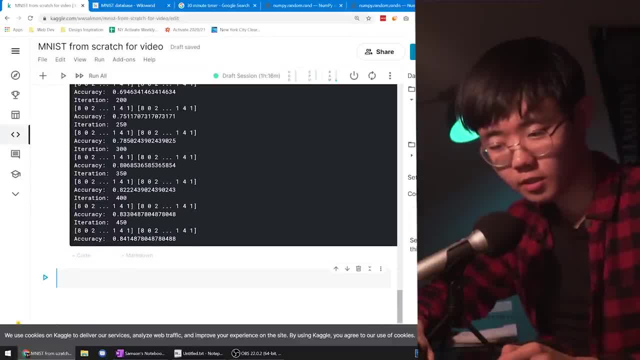 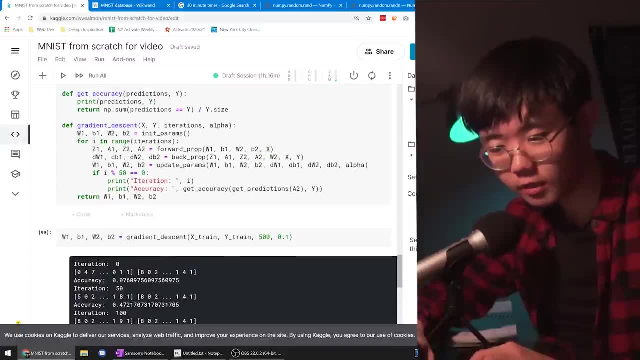 Things like adding more layers, adding more unit cell layers, But 84% for this, for something that we threw together in less than 30 minutes, is not bad. It's not bad. So let's try out a few things. Let's now. 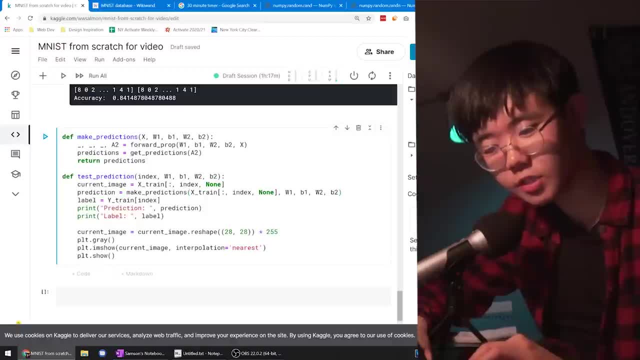 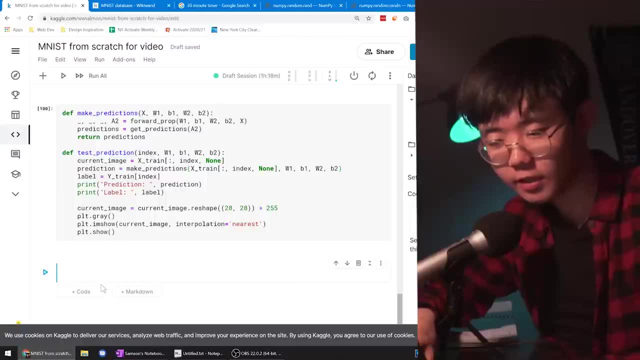 And I'm just going to rip code straight off from my old thing. now, This is just a function to make that prediction and then print out the prediction in the label and then display the image. So once we've defined that, let's do test prediction. 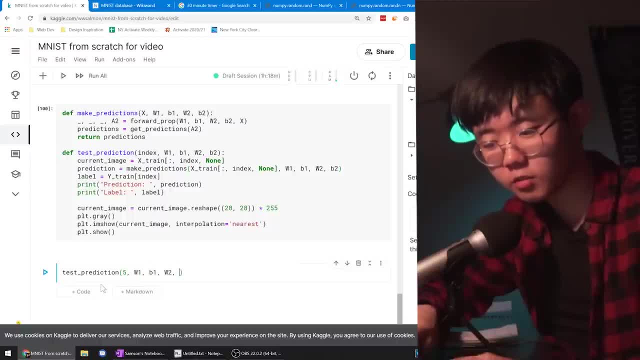 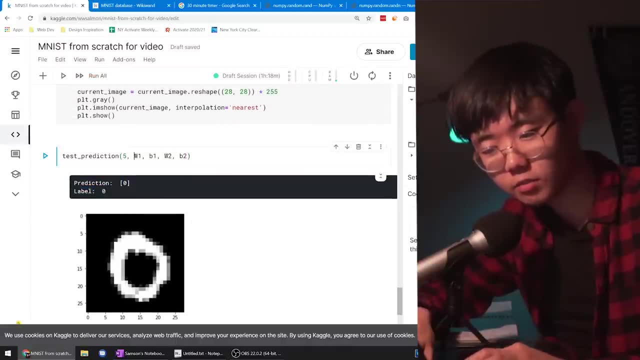 Let's test out just a random number, It doesn't matter: B1,, B2,, B2.. So bang, it's zero. Our model predicts a zero and the label is zero. Let's do the second one. So there we go. 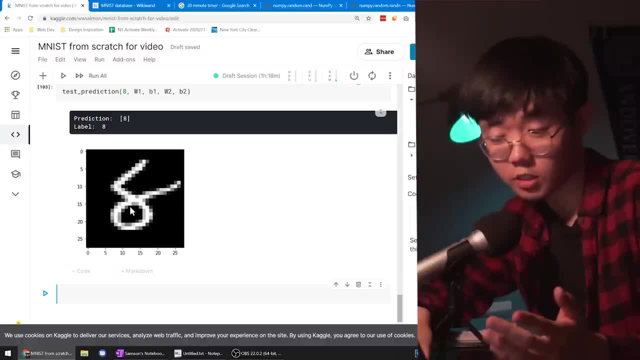 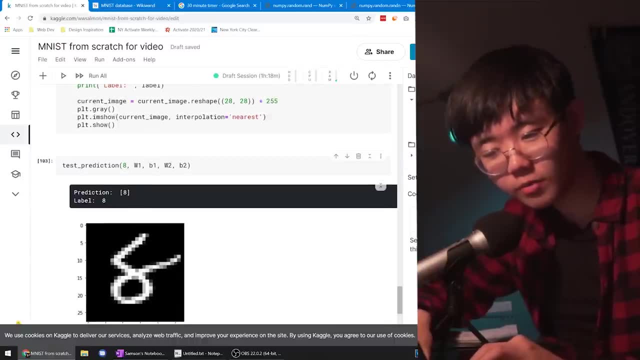 Let's do this one, So yeah. So this is a tricky one. This is a weird. You could see maybe it's a four or maybe it's a five or something weird, But no, the model did it. It's an eight and the label is an eight. 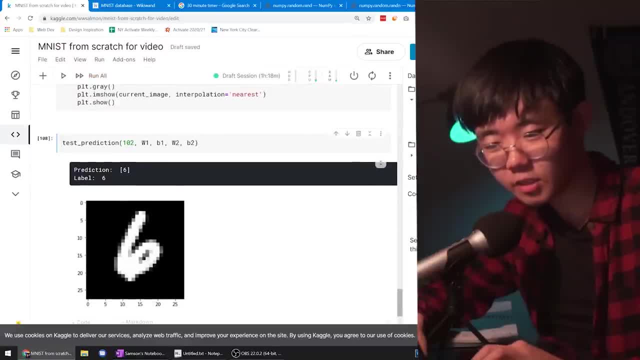 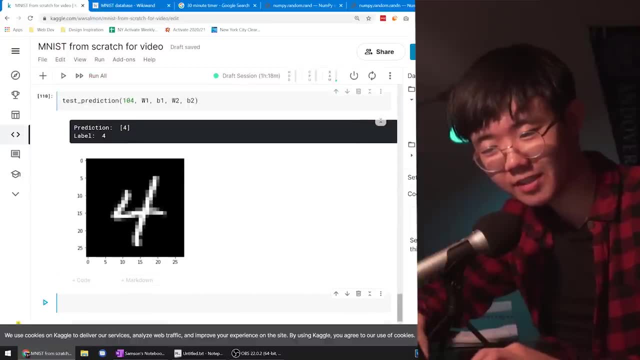 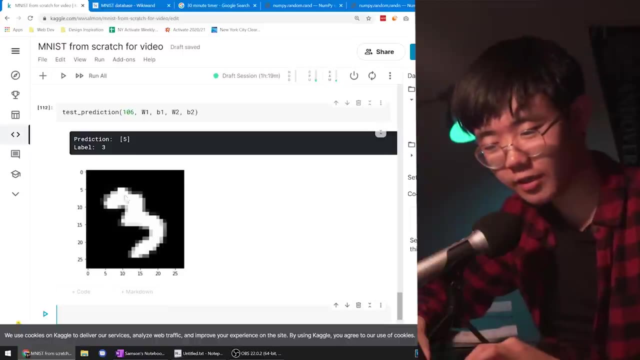 I need to find one that it mislabels, because the mislabels are pretty interesting as well. OK, We are going sequentially in. We're not finding one that it's mislabeled. It's doing really well, Here we go. Here's one. 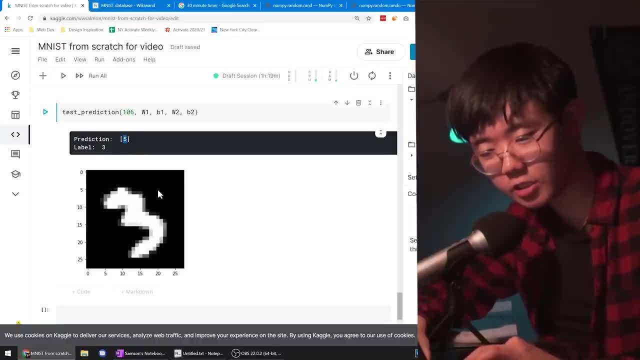 Yeah, So this is a jank three and it labeled it a five, right, Because you can definitely see, like, just like, put the thing here and it's like a perfect five. This is the kind of thing that if you had more layers, if you had more units, you'd. 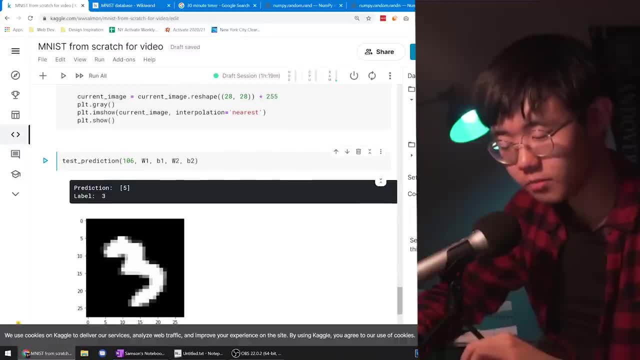 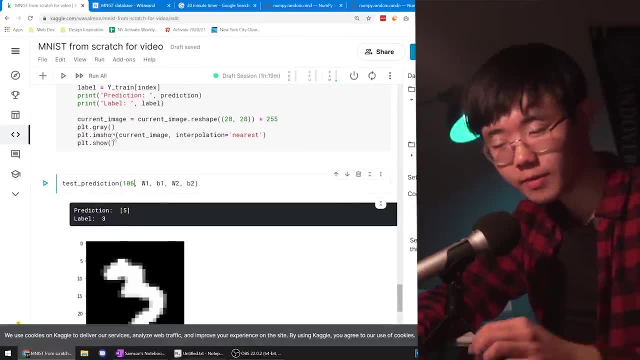 be able to recognize it better that this model wasn't quite complex enough to capture that like basically like a 45 degree rotation here. But you know we went through a good amount without finding one that was mislabeled, So this is definitely a model that actually worked. 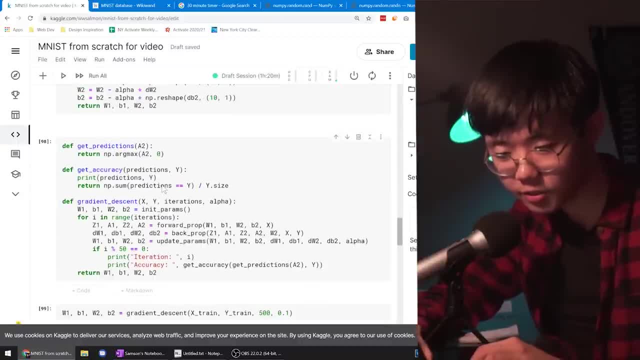 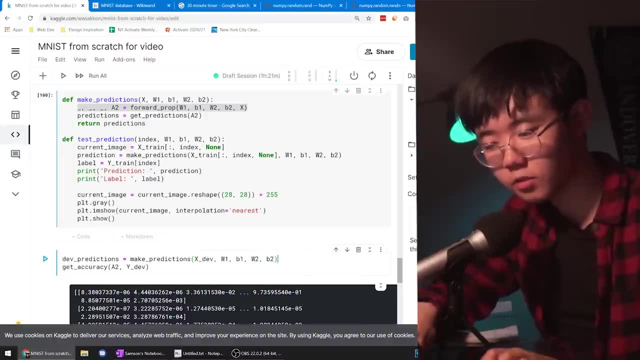 Just to do the last step, I want to check what the cross validation accuracy on this is. Next, dev: If you want to be one to be to be two, OK, And then dev predictions: OK, Let's run that through And OK. 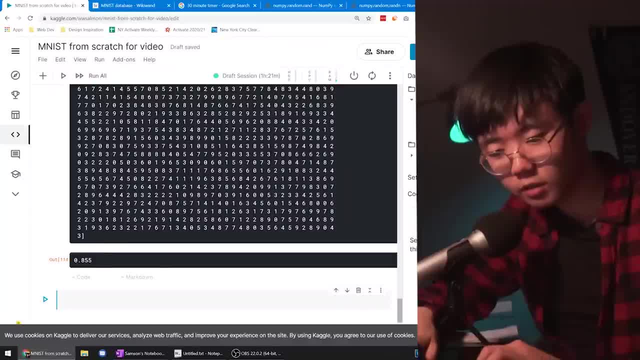 Look at that. That's an eighty six, eighty five point five percent accuracy on the dev set. So that's not the training data. We didn't train on this data. This is effectively testing data Right. We haven't done any optimization for this data. 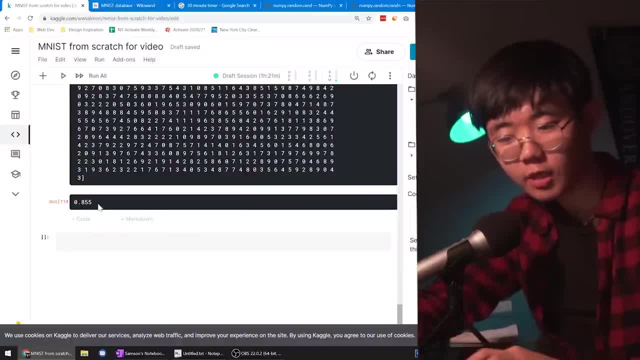 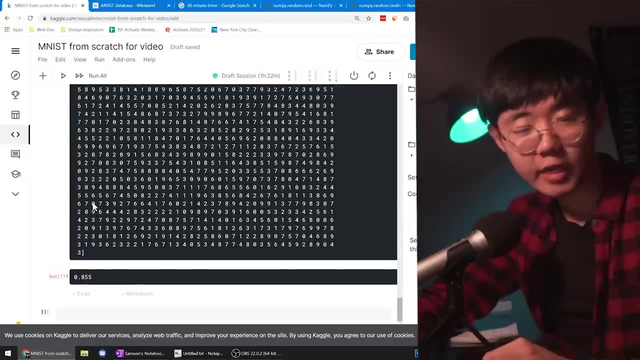 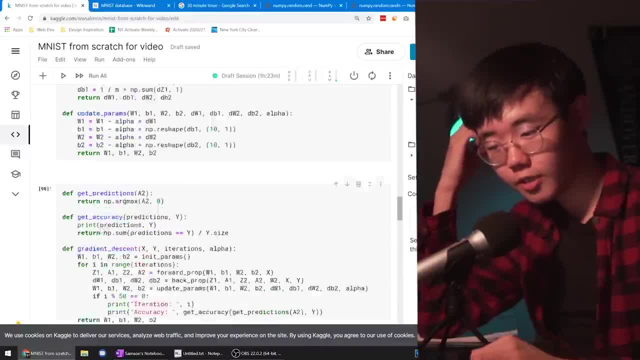 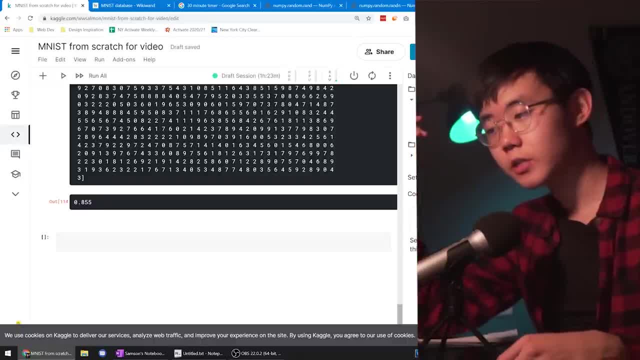 me explain those equations. hopefully it helped a bit. I'll have a link in the description to an article or blog post that I'll put up just with all of these notes. I'll have a link to this notebook so you can look through all the code. 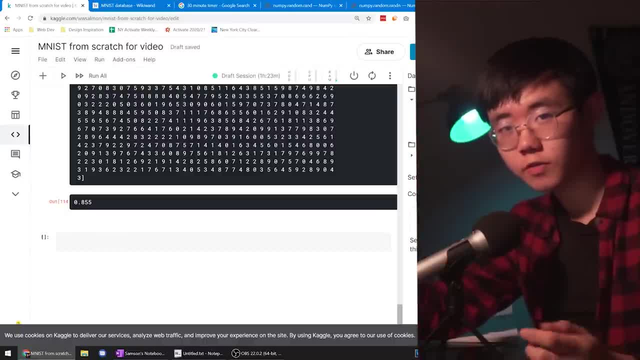 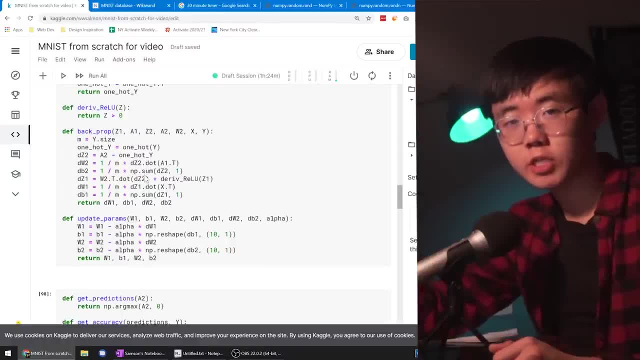 You can look through all the equations. You can figure anything out for yourself if you so desire. There's a lot of other stuff to explore: implementing manually, right So things like regularization, different optimization methods, right. so instead of just gradient descent, there's gradient descent with momentum, there's rms prop. 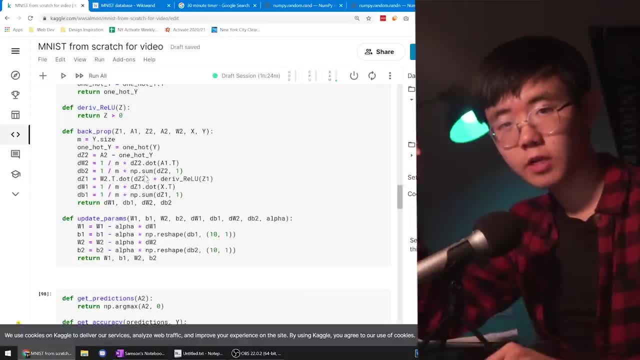 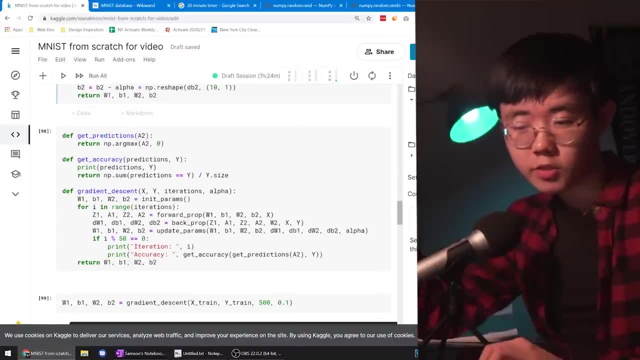 there's atom optimization, which are all just variants of gradient descent and they're fairly simple to implement. but it could be interesting just to implement that yourself and see what the impact is. yeah, this is a fun exercise. it's always satisfying to see the accuracy go up like that. 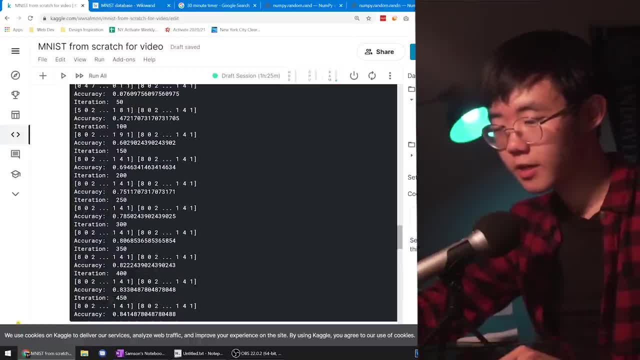 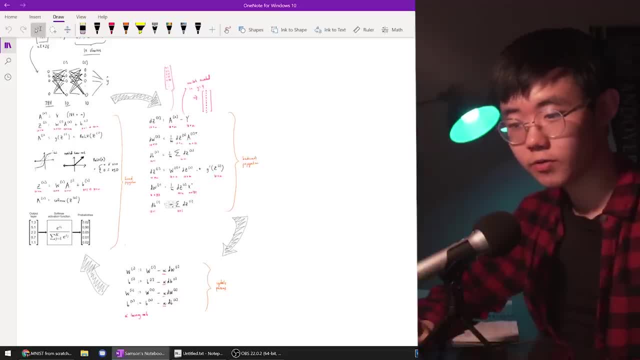 it's satisfying to see on like a model that you train using like charis tensorflow, and it's it's all the more satisfying to see on a model that you built yourself. that'll be it for this video: just a simple demo of how you can build out all the math that's on this screen here. i hope this.